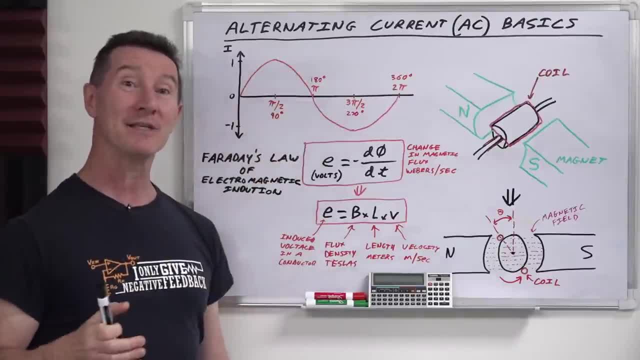 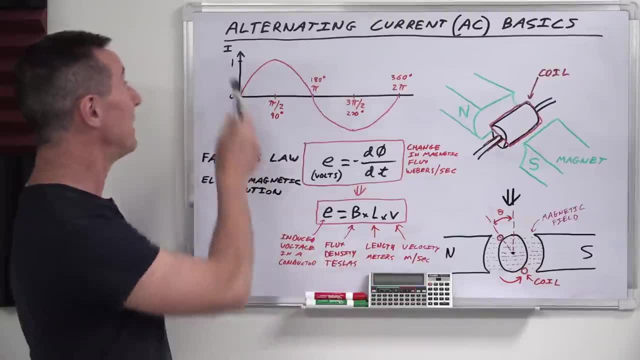 So let's have a look at alternating current basics. So what is alternating current compared to DC or direct current? Well, it's obvious, It alternates polarity. If we've got our waveform like this, DC would just be like: this is 0 volts, this is 1 volt, or we've got current here. 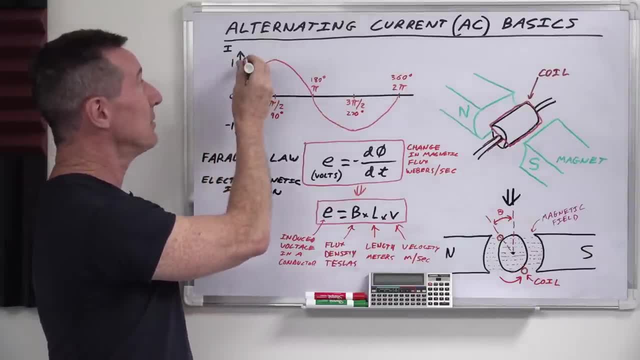 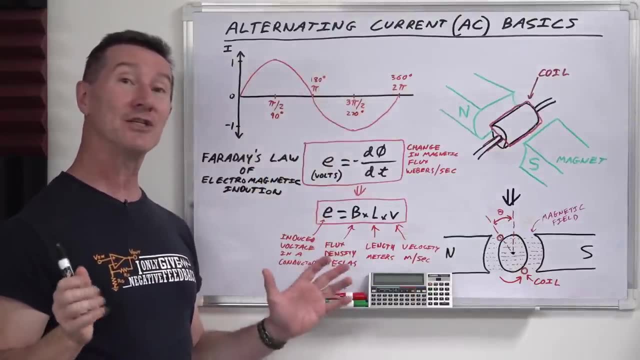 So let's say 0 amps, 1 amp up here, DC direct current would be just a straight line like that, It'd just be 1 amp. But alternating current, it changes direction. It's positive up here, in this case positive 1.. 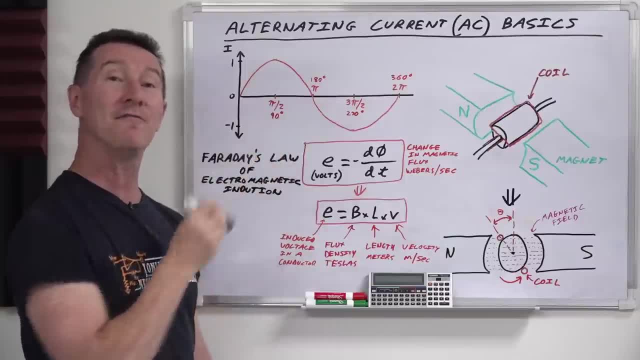 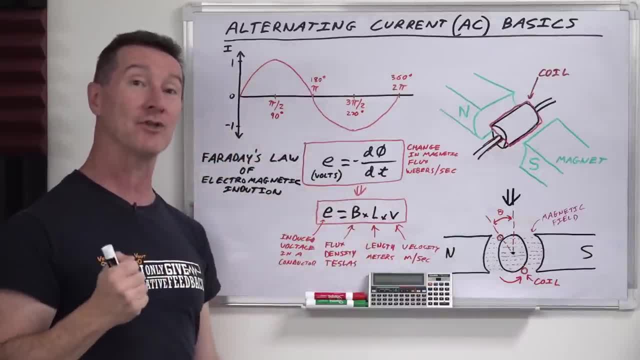 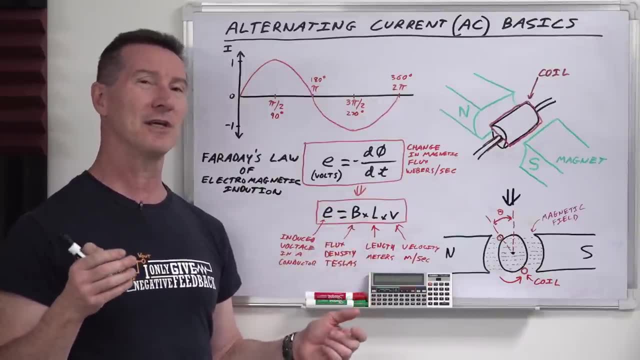 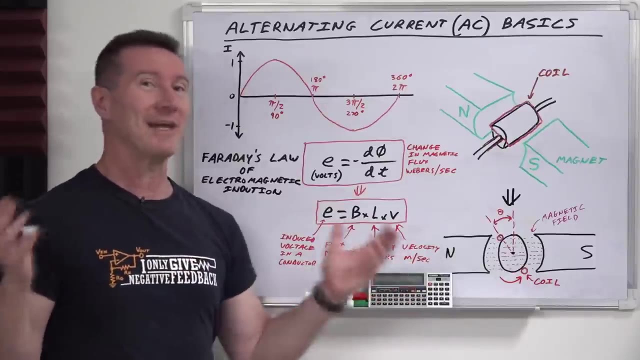 that the current, the electron flow, actually changes direction and that's pretty much the definition of ac or alternating current, which is confusing because you can go ac voltage and it's like well, alternating current voltage. that doesn't make sense, but that's the terminology, ac voltage. you'll 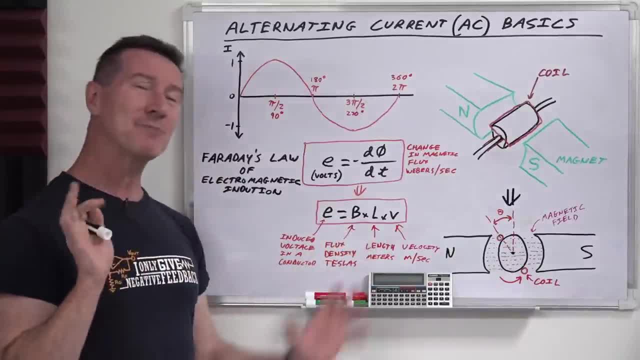 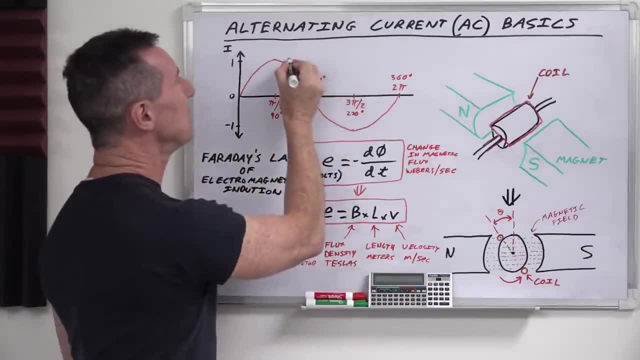 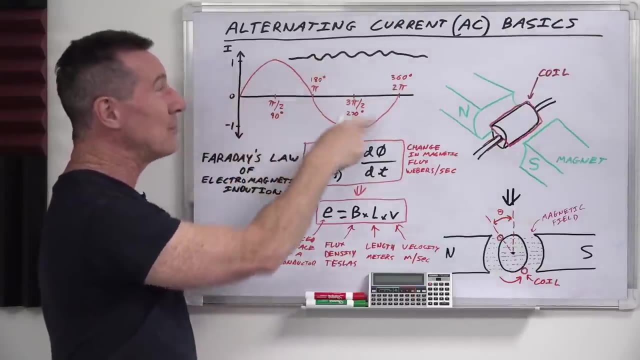 find lots of stuff like that in engineering. but- and that's pretty much the definition of ac- is it really has to change polarity like this? if you've just got dc up here which might have some ripple on it like this, that might look like alternating current, but it's still direct current with ripple. 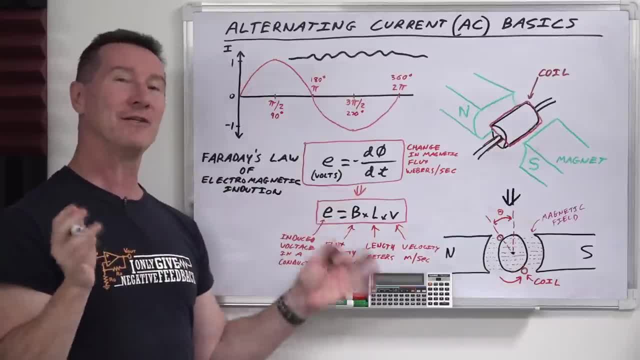 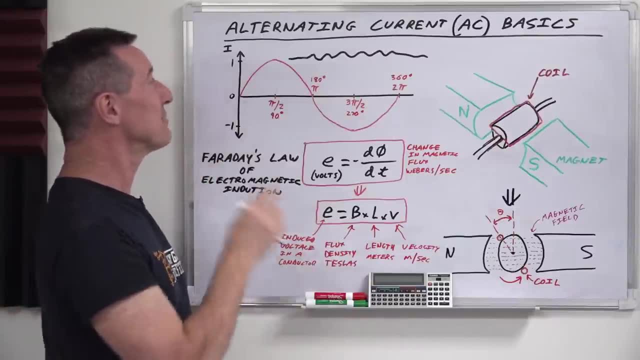 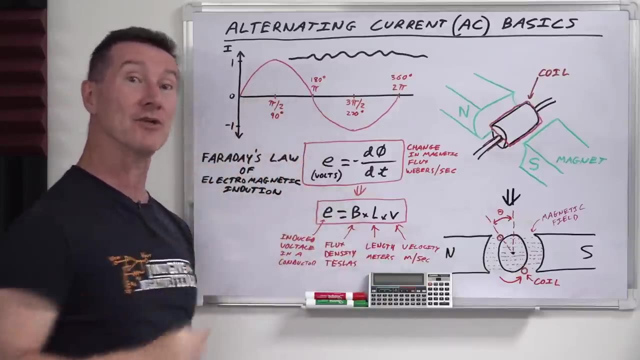 and, yeah, flame wars in the comments down below the difference between is this actually ac and is it dc. anyway, get into the details of this, but suffice it to say for this video, we're talking about alternating current, that's physical current, physically changing direction, and this is super important. 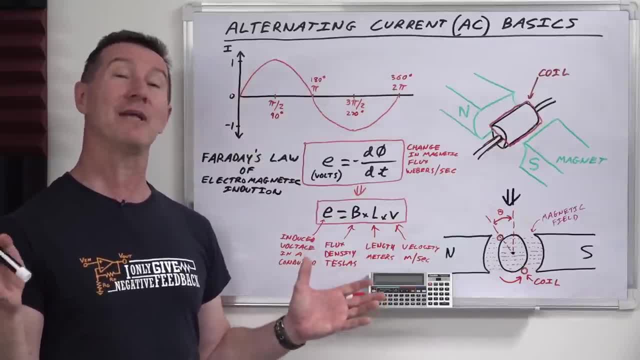 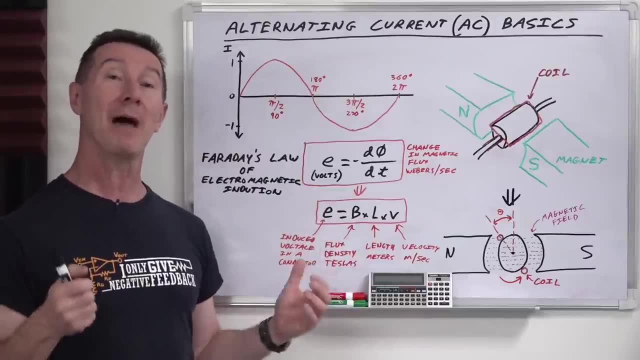 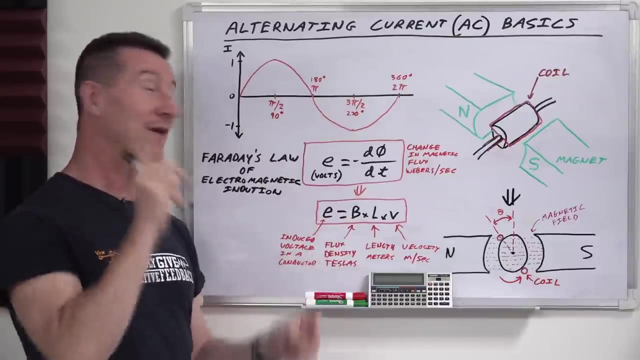 theory, because most of our power generation and our telecommunications rf signal transmission. this all happens in the ac domain and this all happens with the sinusoidal wave like this. and there's actually something very special about the sinusoidal wave, as we'll go through in a minute. 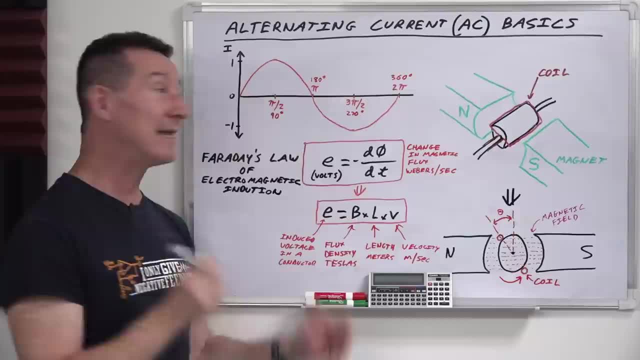 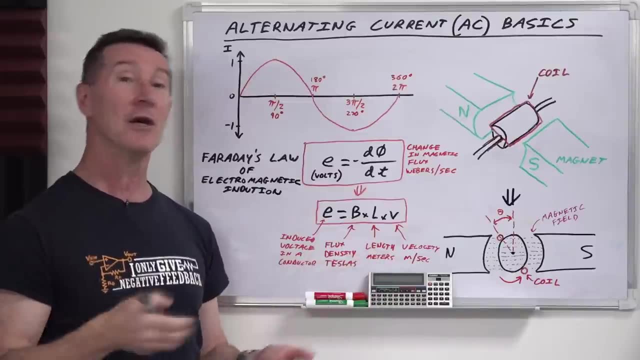 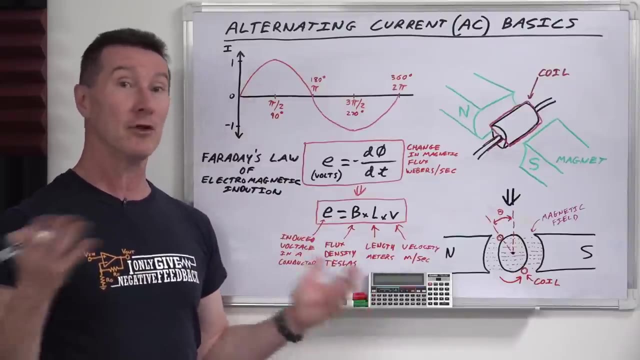 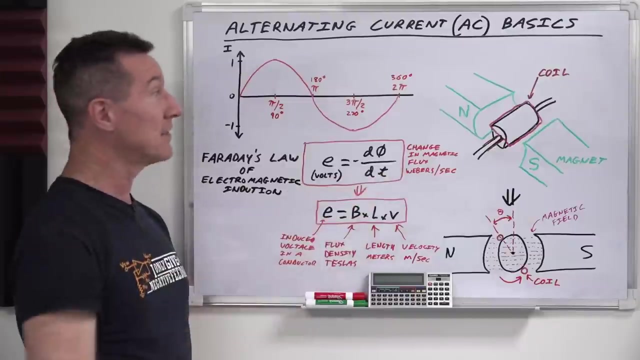 the sinusoidal wave shape like this comes about naturally in rotating magnetic fields, like you get in generators, which is used for most of our power generation, be it uh wind turbine generators, hydro power generators, steam power generators, which are also nuclear. nuclear energy just heats up steam, basically, which then drives a, a turbine, which drives a generator like this and that. 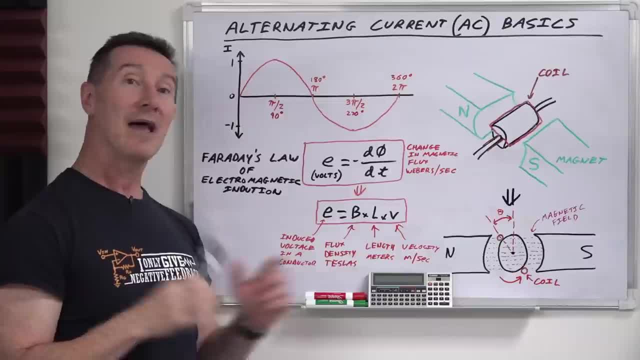 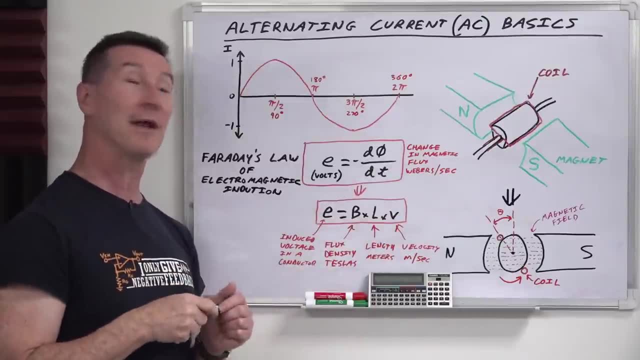 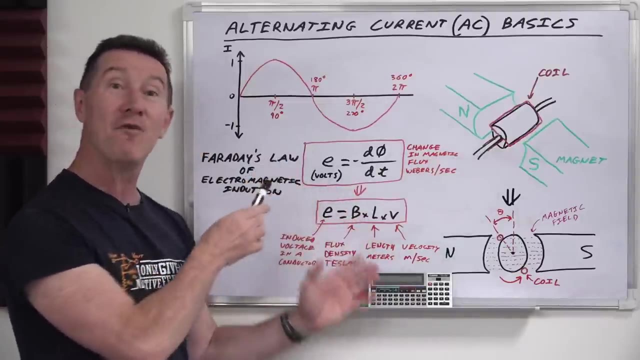 generates always a sinusoidal output. actually, you want as close to a perfect sinusoidal output like this as possible on a generator for reasons where that we're going to get into. so we're going to look at how a basic generator here works and this brings us back to a formula you've seen before in. 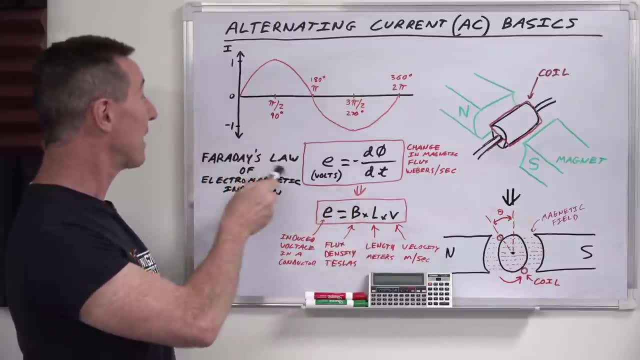 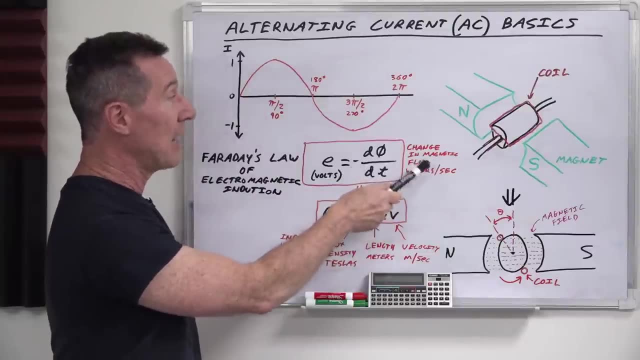 even dc fundamentals when we talked about inductors, faraday's law of electromagnetic induction, the induced voltage in volts is uh, negative, uh. the chain which is lenzer's law- won't go into details, watch previous videos- the change in the magnetic flux in weber's per second. 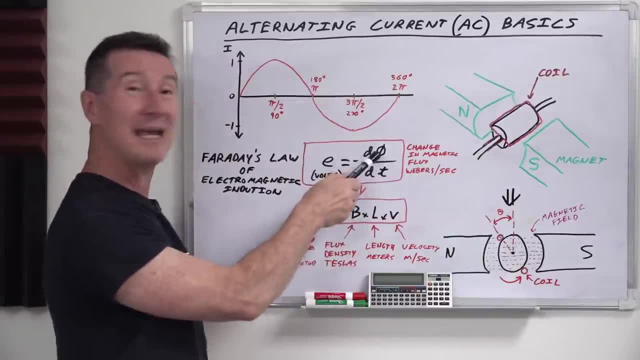 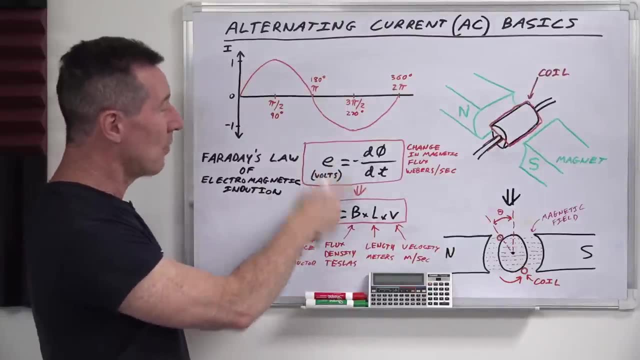 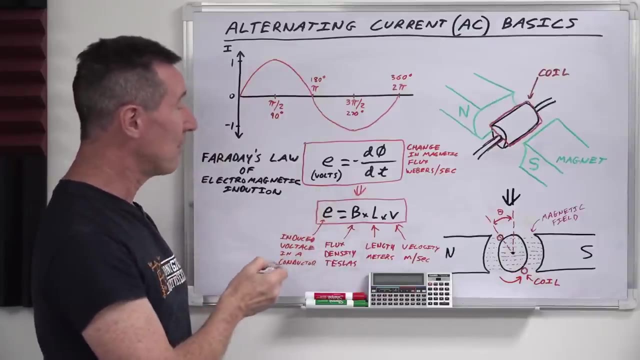 so basically defy dt here just means the change of magnetic flux over time in weber's per second, and that's it. and then i won't derive how we actually get down to here. but basically this formula here you should pretty much remember along with faraday's law. this is the formula. 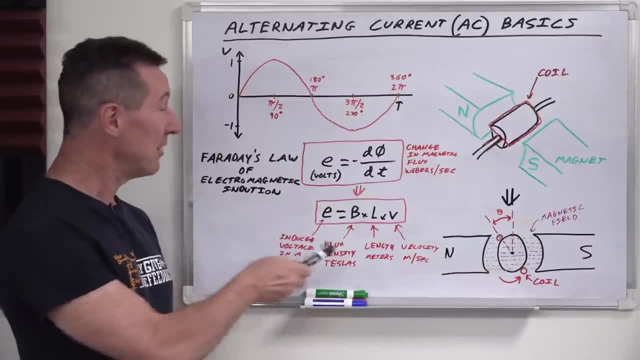 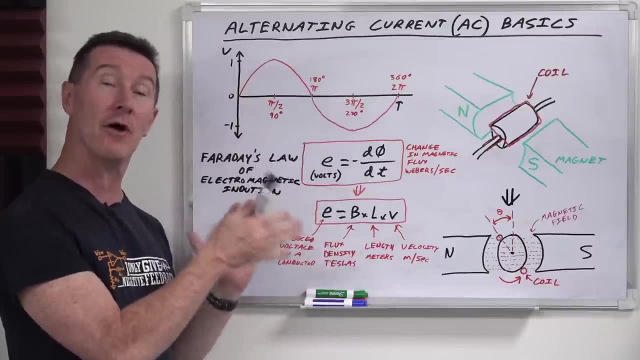 for the induced voltage in a conductor in a magnetic field, and it's equal to the flux density in tesla's b multiplied by the length of the conductor at 90 degrees to the magnetic field in meters, multiplied by the velocity of the conductor through the magnetic field. 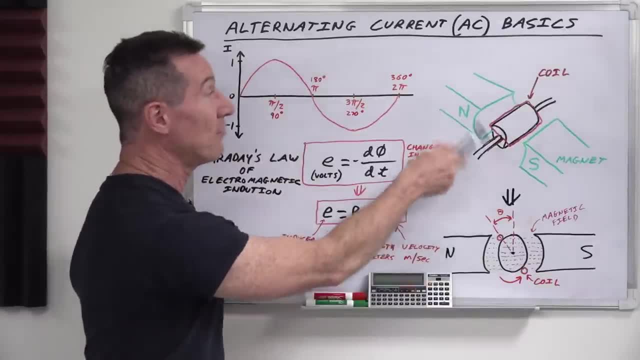 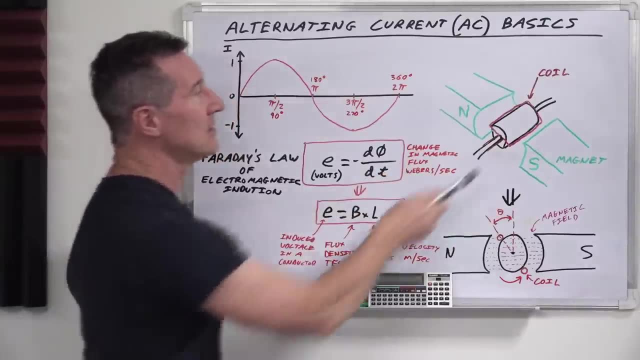 in meters per second, simple. and of course, we've got all that stuff inside a generator like this. so let's have a look. we've got a north pole of a magnet, south pole of a magnet like this. we've got a shaft in there like that which contains a core, and that red uh part around there is just a single. 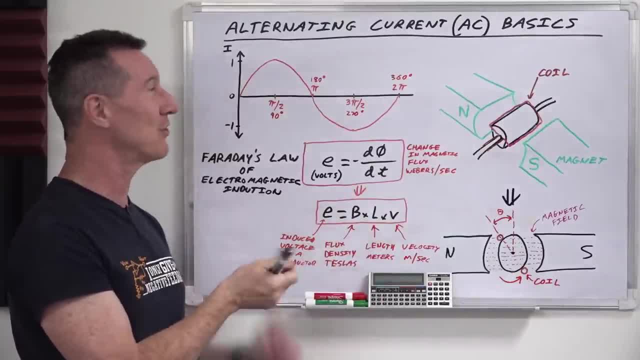 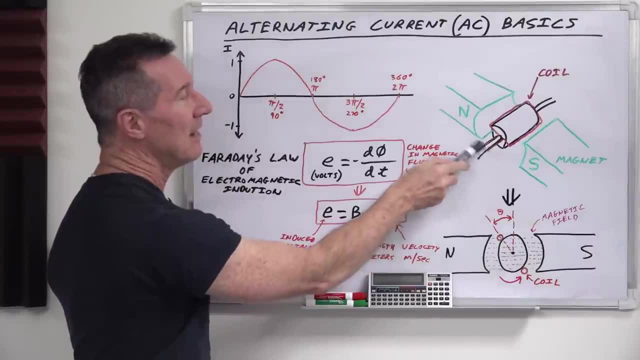 turn coil. of course it can be multiple turns. you wouldn't have a single turn coil in there, not very efficient, but we'll run with a single turn for today and the wires come out here like this. now i won't get into details of how the power actually uh gets out of there. i go into, like, the mechanical slip rings. 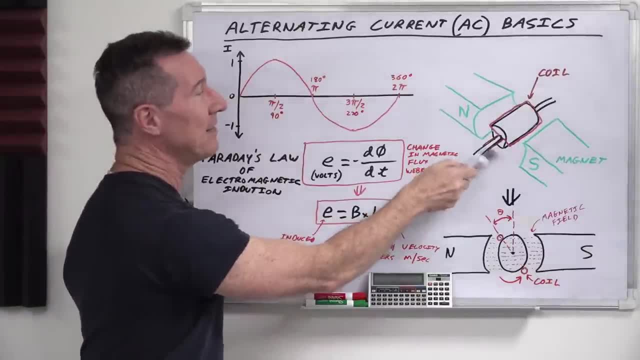 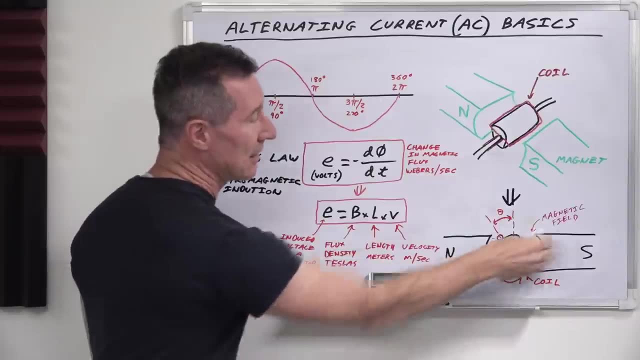 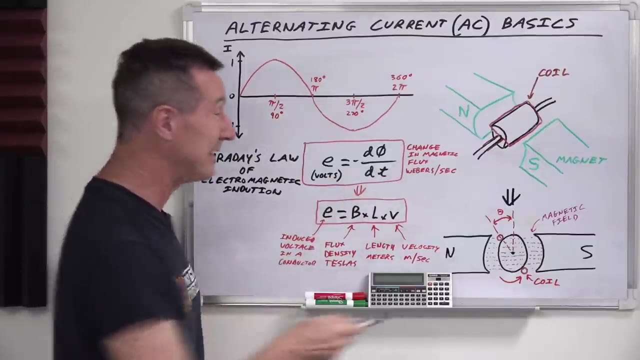 and everything like that doesn't matter, okay. basically, voltage current comes out of the coil like this as it rotates in a magnetic field and if we have a look down here, this is like a side cross section of this 3d model up here. please excuse the crudity of model, didn't have time to build the scale or to paint it. um, at north and. 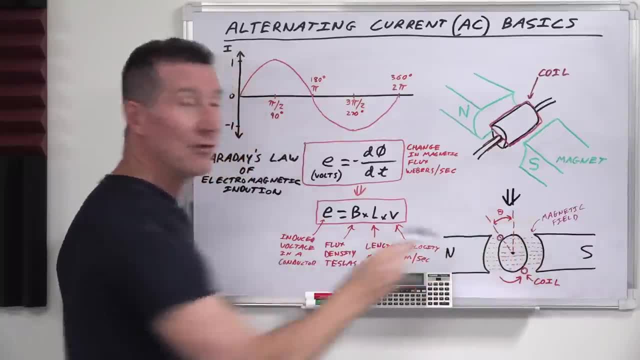 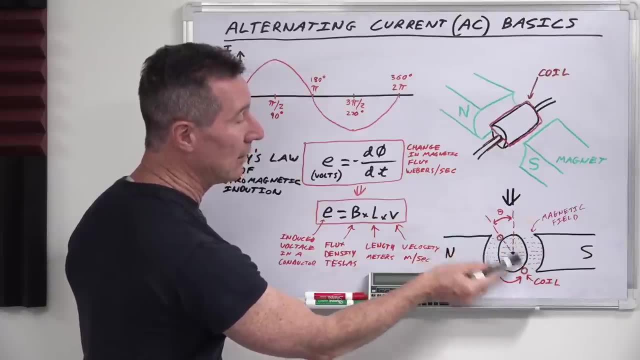 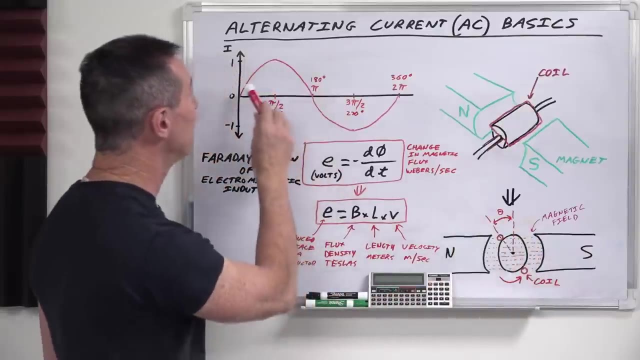 south pole. here we've got a uniform magnetic field through here- let's just assume that it's a uniform magnetic field. and then we've got our coil here and here like this, and the coil will rotate through the magnetic field like that and go around and around and around, and this will actually 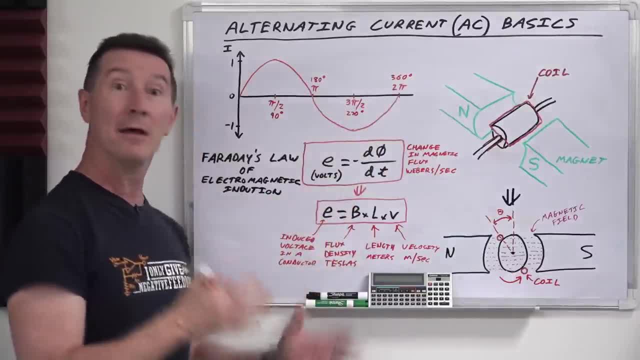 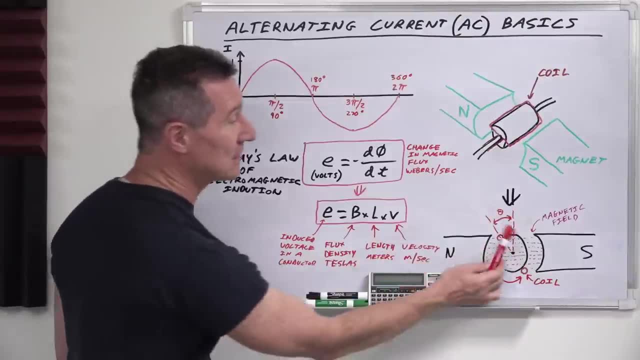 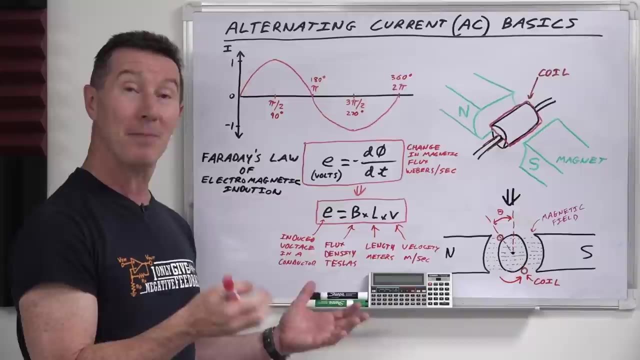 produce a sinusoidal wave shape. how does it do that basic trigonometry you learned in school? if we uh take, like the vertical axes, like this as the the angle of the coil, like this is theta here and theta is the angle, and of course you know your basic trimming trigonometry, it's just sine theta. 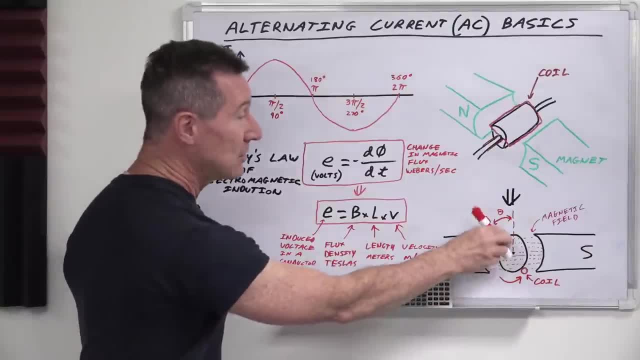 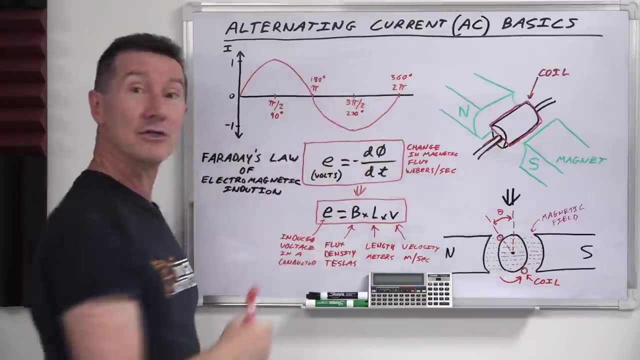 is the angle through that field. so as it goes through it actually naturally develops. assuming you've got a uniform magnetic field and everything's hunky-dory, you get a sinusoidal wave shape out like that and when the coil is right in the middle of the coil it's going to. 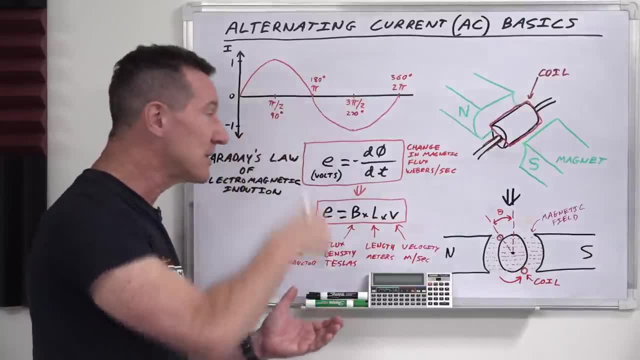 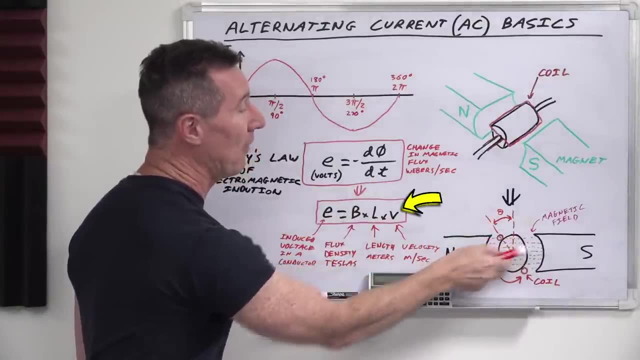 move in the horizontal position like this: this is the actual maximum velocity through the magnetic field. like this, it's at its highest velocity at this point, so at 90 degrees, like that. this is when you'll generate your peak voltage, here and here, like this, depending on which orientation it is. 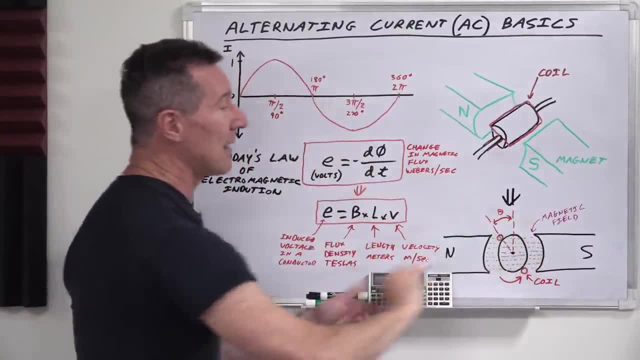 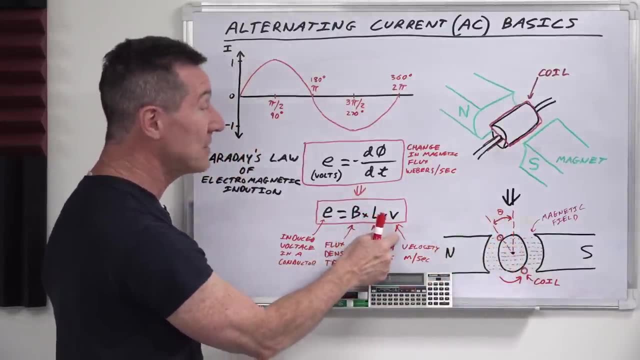 depends on which, whether it's positive or negative peak, but when it's up right at 90 degrees, like this, it's not. there's basically no movement through the magnetic field. the velocity drops to zero because it's not going through the magnetic field. the magnetic field's 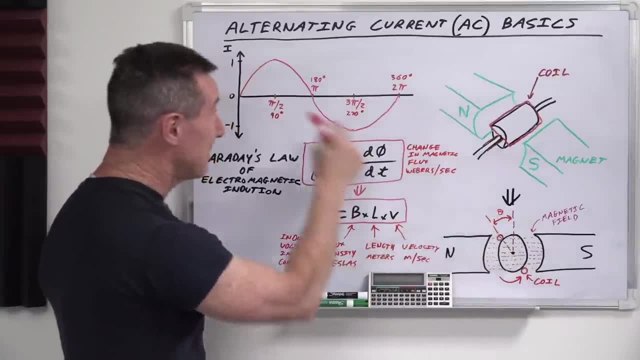 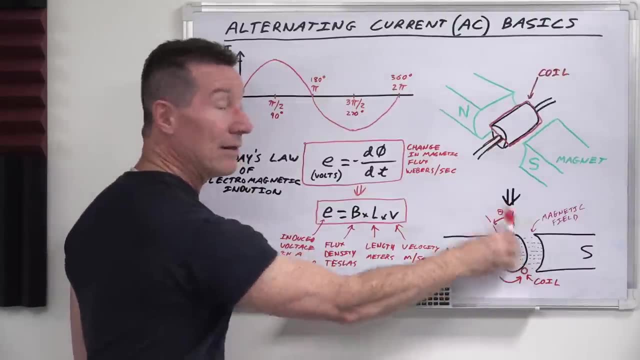 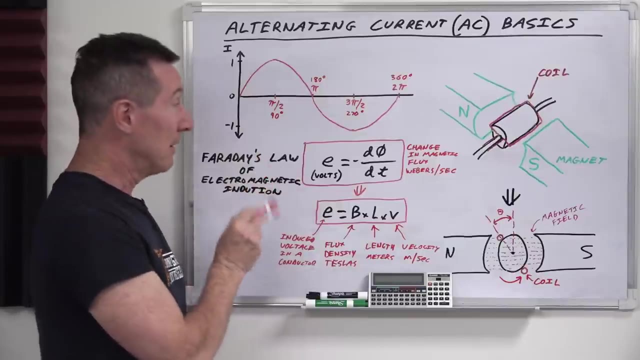 going in this direction. it's basically: it reaches a point where it's it's zero. so here here, here it's basically generating nothing when the coil is vertical, like that. pretty simple. but that's your basically basic formula for induced voltage in a magnetic field. so basically our maximum voltage. 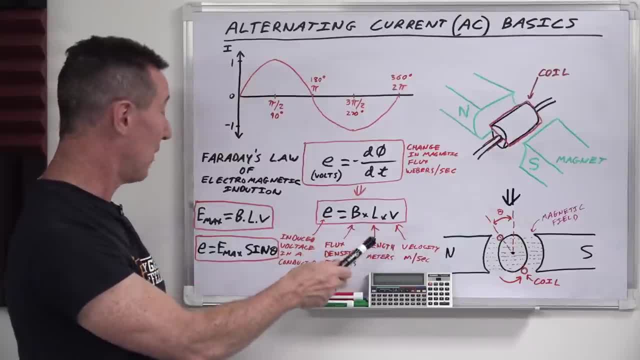 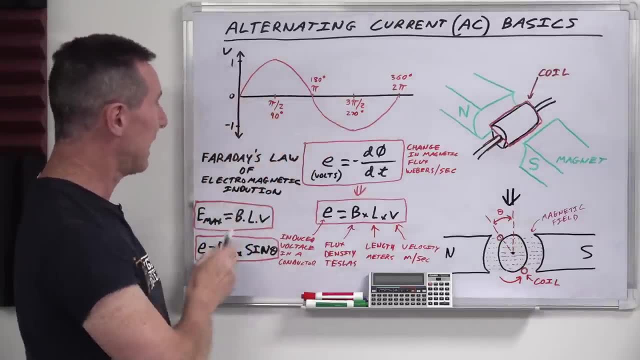 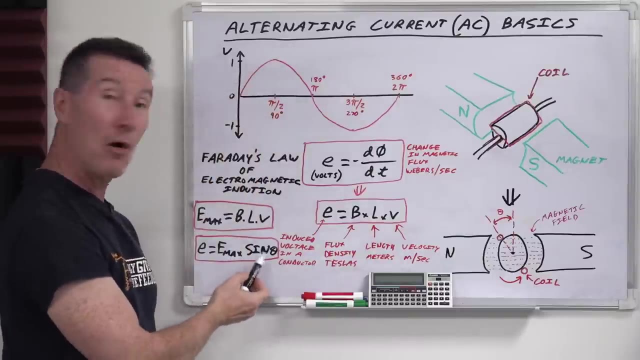 here our peak voltage we're going to get is b times l times v, so the instantaneous voltage here. so let's well, this could be e voltage here. the instantaneous voltage at any point in time here equals e max, which is the maximum- assuming it's like one up there- multiplied by sine theta, the angle of the coil in the magnetic field. so 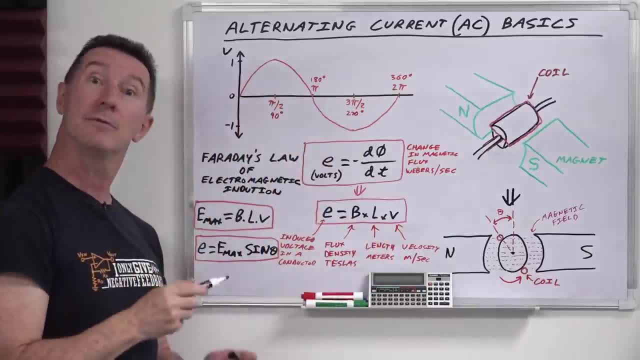 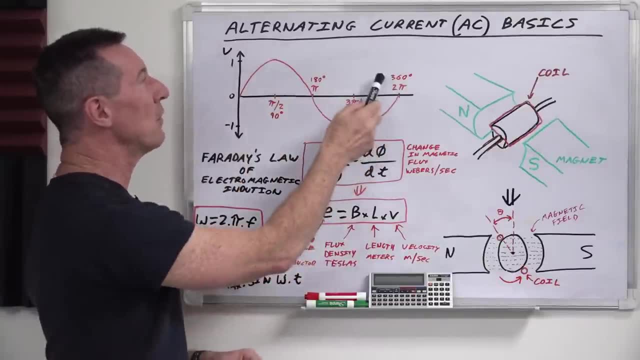 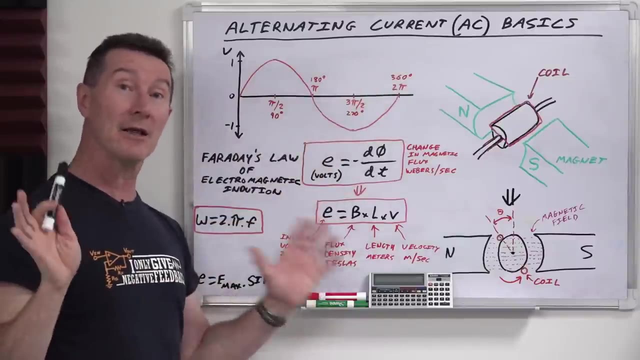 therefore, you end up with that sinusoidal shape, simple. so in basic maths, when you're talking about sinusoidal waves and cosine and and tangents and everything else, you might talk in terms of degrees like this: so zero degrees, 90 degrees, 180 degrees, 360 degrees, and in electronics we do talk about, in engineering we talk about. 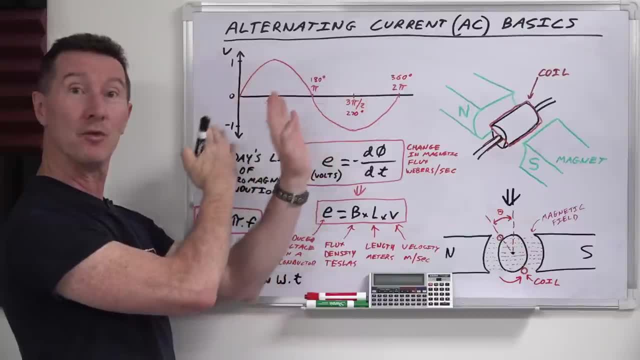 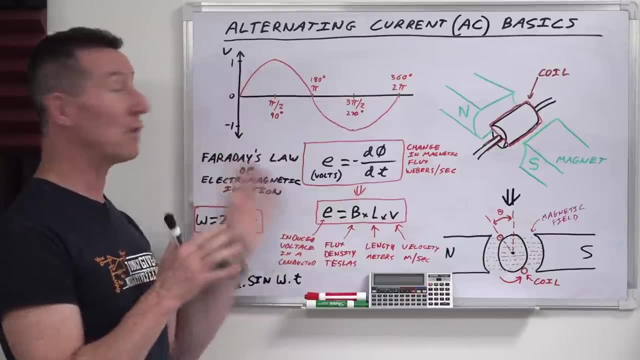 uh degrees in terms of phase difference. so if you have two waveforms and they shift like this, we generally talk in terms of uh degrees. but what's more helpful to use when it comes to talking about ac stuff is to talk in what's called angular frequency. so we use w to represent that which is. 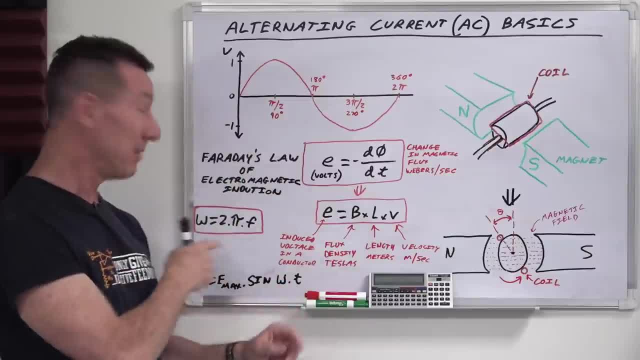 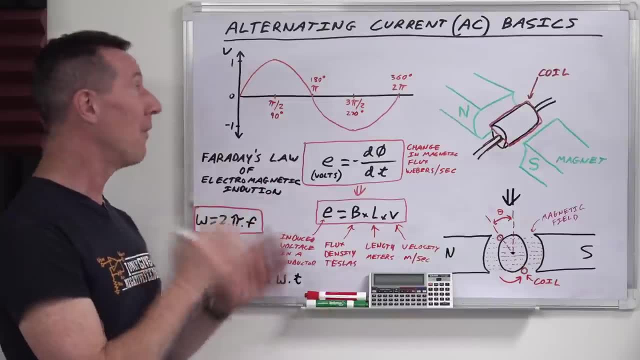 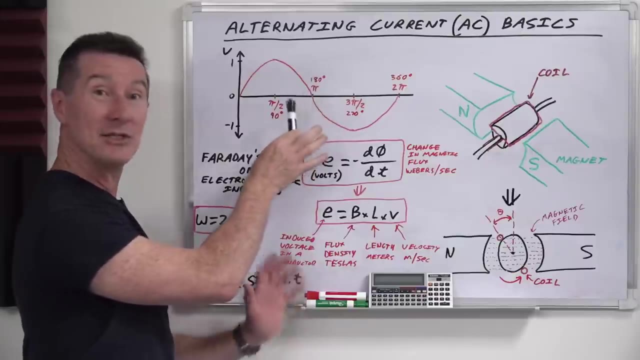 actually uh, omega in the greek alphabet it's not just the ohm symbol, it's also the little w thingy anyway. greek alphabet- rubbish anyway- equals 2 pi f, so we talk about this in terms of pi. so 90 degrees is actually pi on 2, 180 degrees is just pi and 270 degrees is 3 pi on 2 or however you want to. 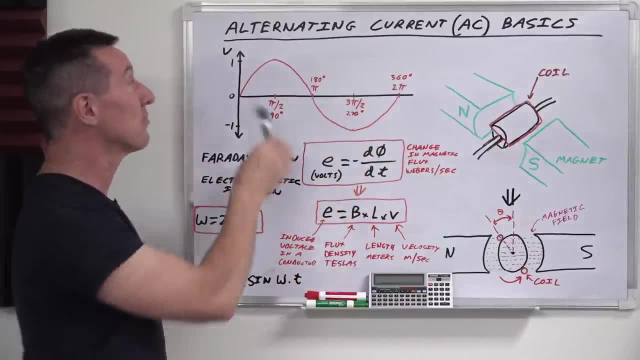 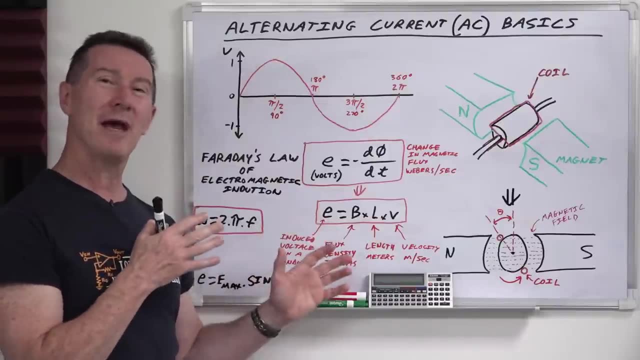 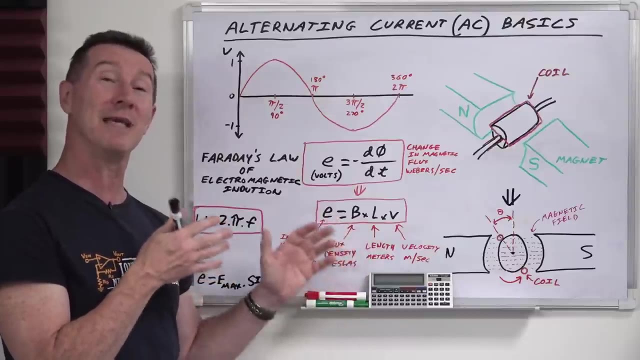 represent that, and 2 pi is 360 degrees, ie a full cycle of an ac waveform like this, because it's not just one of those kind of like two separate wave types, but it's a whole. another thing that's very, very important to talk about as well, and we'll talk about that in a minute. 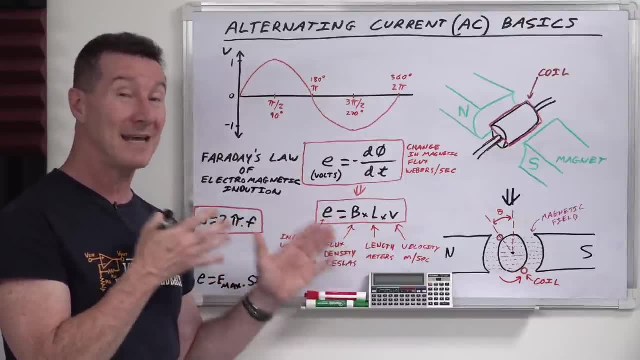 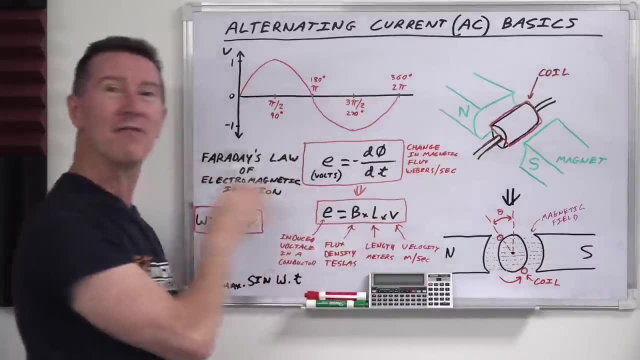 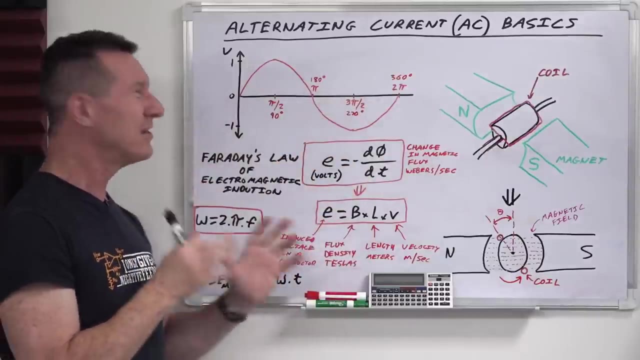 but as one thing i actually didn't point out before is like another definition of ac or something that it needs to include this to be like deemed to be ac, and this is what differentiates it from, uh, the transient analysis. in dc, you just have a single transient, like this ac actually has to have. 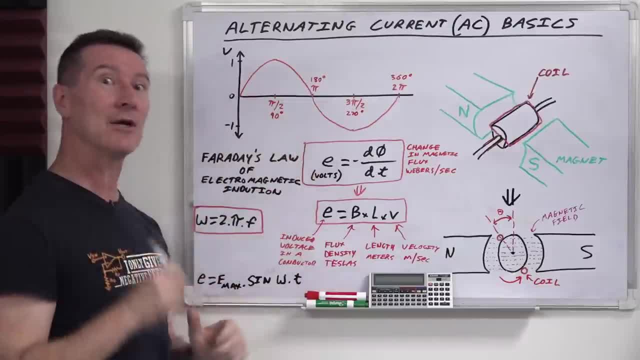 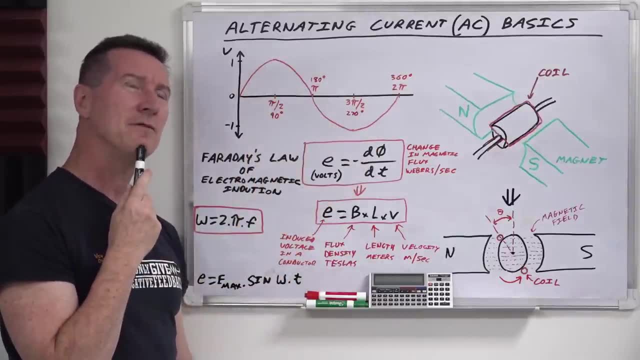 a frequency, it's got to have a period and it's got to in quote marks. so yeah, it's. it's got to be more than just if it's one cycle. hmm, if a tree falls in a forest, do you hear it? and if you've only got one cycle, is it still? ac comment down below. 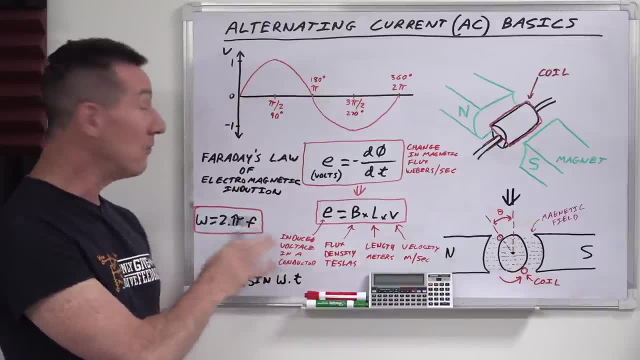 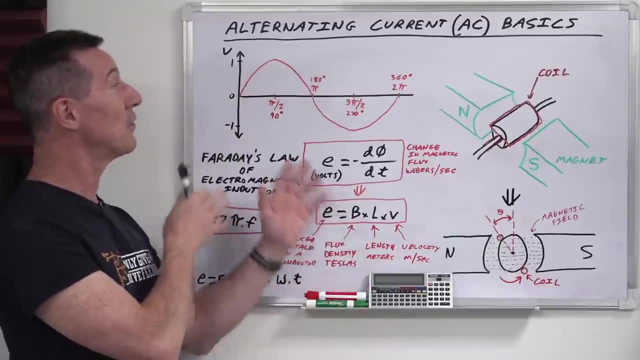 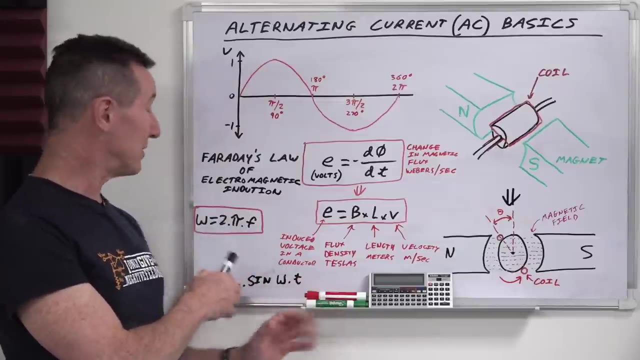 anyway, the angular frequency is 2 pi f and you'll find this 2 pi everywhere in electronics and 2 pi f is very important and in this case we're talking about angular frequency like this instead of degrees. anyway, this is in units of radians per second, so, and we can do once again. 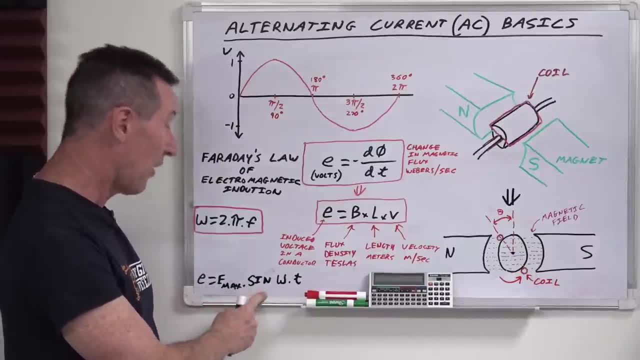 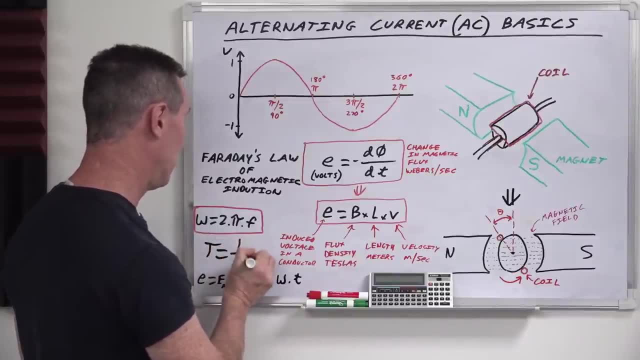 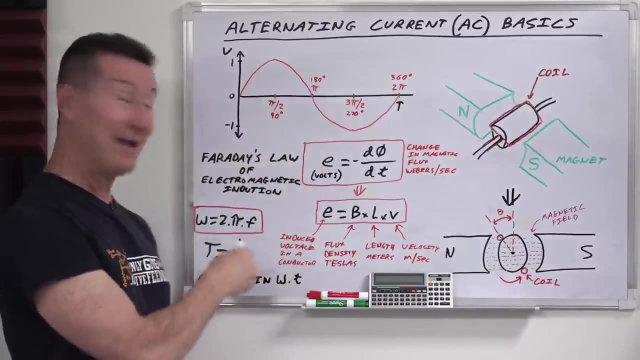 the instantaneous voltage, e equals e, max times, c, uh, sine, omega t, like this. and then, if you run it through the wash, t equals one on f, and with t being your time period, like this. and well, that's one of the most fundamental equations in all of electronics: how to convert time into 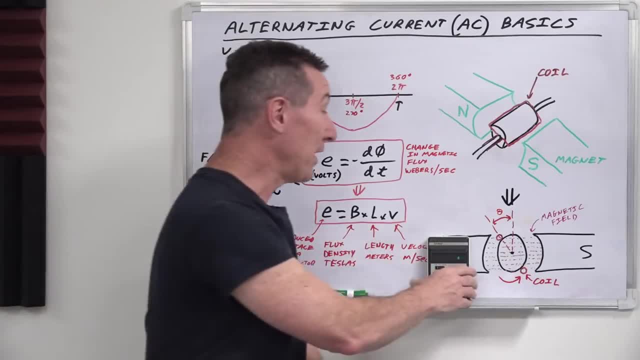 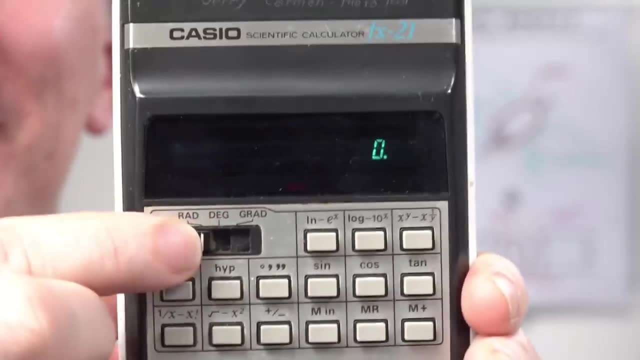 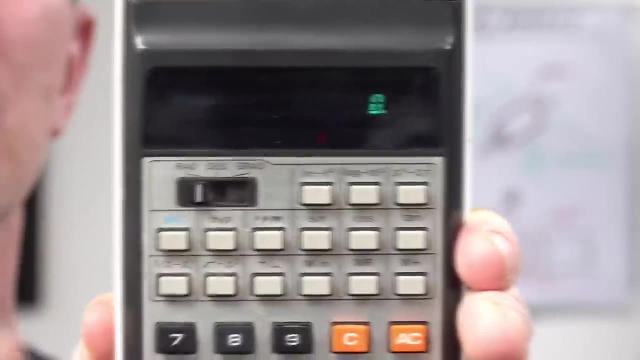 frequency, it's just inverse, and this, by the way, is why your confuser here almost certainly has a degrees and radians and gradients button, gradients and some weird french thing that surveyors might still use, i don't know. degrees and radians mode, your calculator's got it. 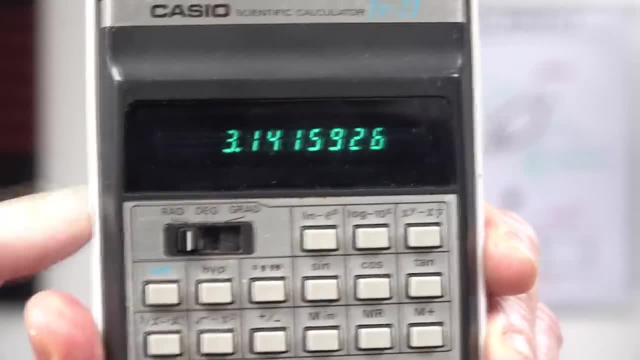 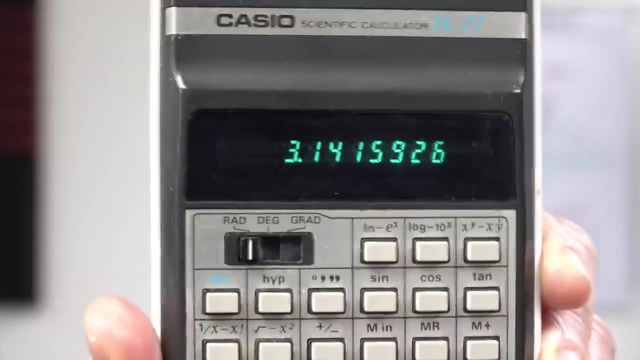 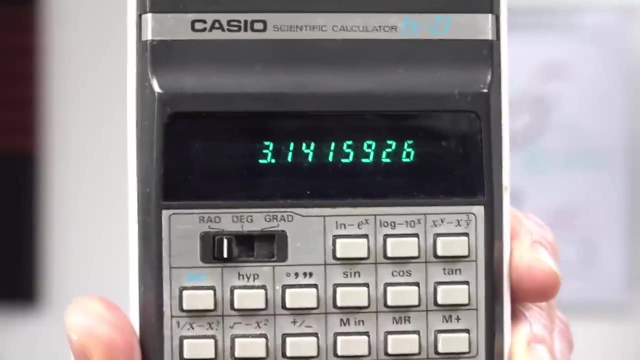 guarantee it. that's what it's for. so that's what it's for on your calculator: degrees, radians or gradients, which is like 400 gradients for one uh, one time period, one t, one turn of your generator is 400 gradients anyway. radians, beauty. so if we do pi. 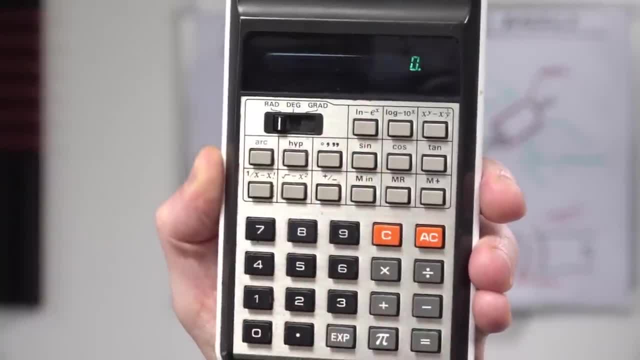 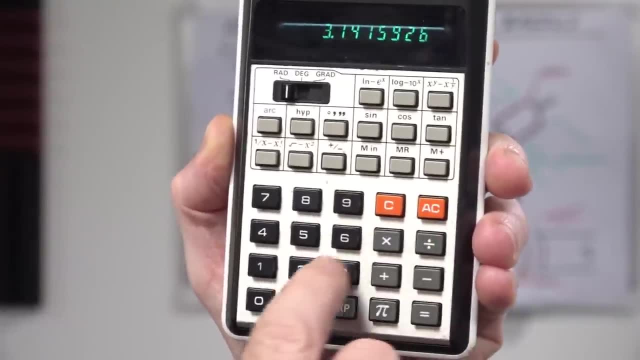 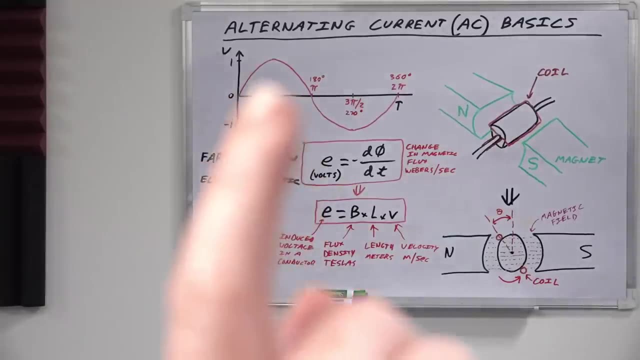 on our calculator in radians mode like this and get the sign of that, it's zero because it's in the middle of the waveform that we saw there. but if we do pi divided by two equals and then sine, ah, it's one because that's when our waveform peaks, right up there, beauty, and then three times pi. 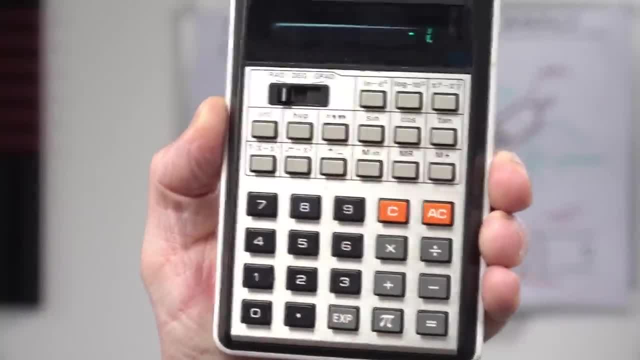 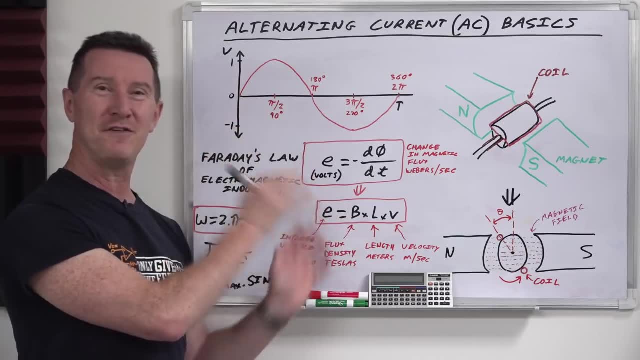 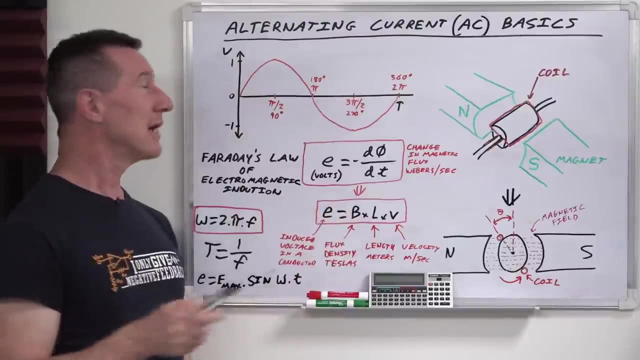 divided by two equals sine minus one, the maths works. and once again, with all this stuff you can really go down the rabbit hole to the physics side of things and advanced mathematics of it and everything, and it's like nah. but anyway, let's get on to the importance of the sine wave and more. 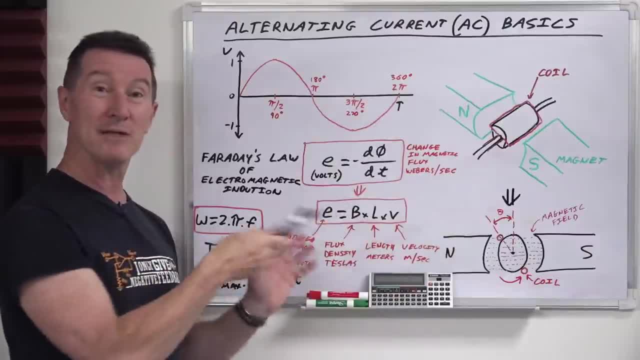 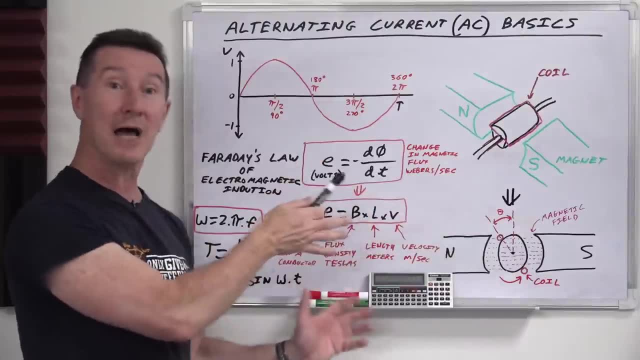 circuit theory related stuff, because that's what we're going to be talking about in the next video. i know that, like motors and generators, might be boring, but it's important that you know where that sinusoidal wave shape can come from physically- and it does in the real world, you know. 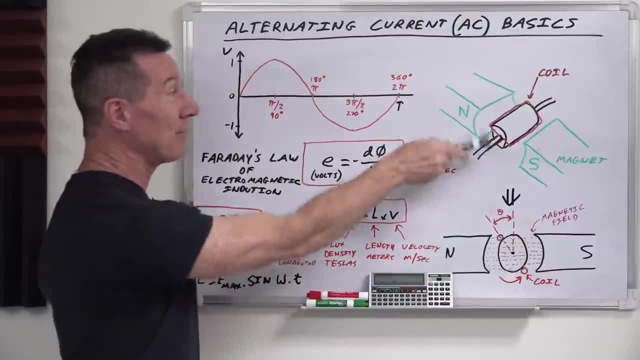 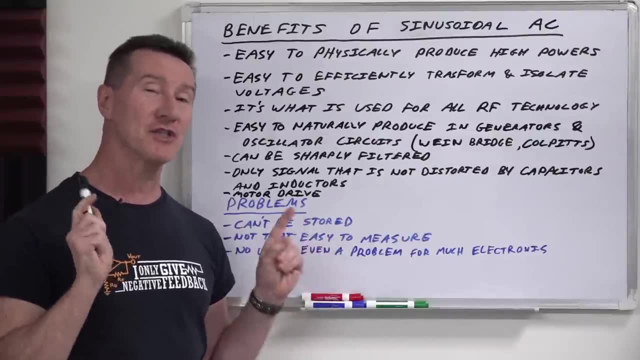 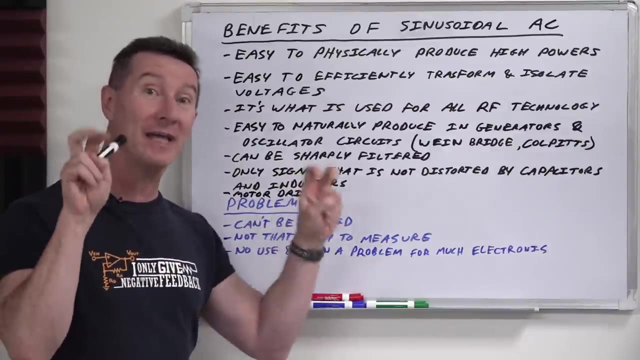 probably a majority of the power that comes out of your powerpoint was generated with a gen, with an ac generator like this. so i mentioned before specific benefits of sinusoidal ac, so let's take a look at them. and this basically applies to sinusoidal shape acs, because it's the ideal ac. 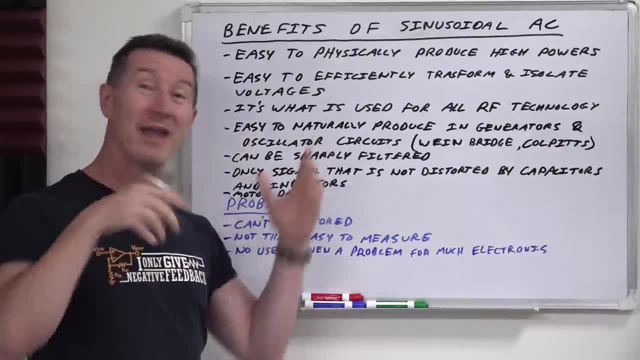 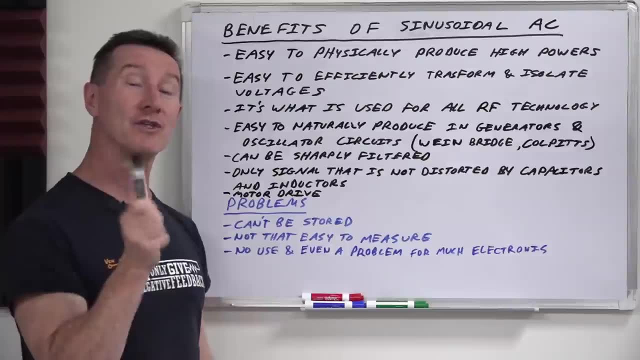 waveform. sure, you can get square waves which are ac, and you can get triangular waves. you can get all sorts of, you know, pulse width modulator waveforms which can be ac and all sorts of stuff, but in particular sinusoidal ones have specific benefits. let's take a look at them. it's easy to physically 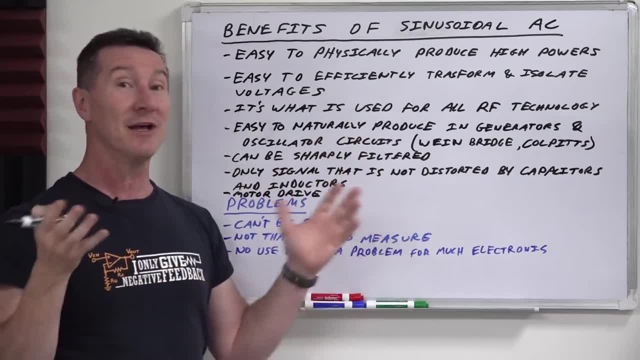 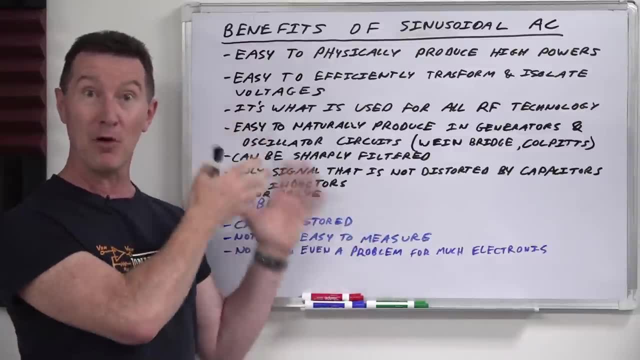 produce high powers. as we looked at those generators, this is how the vast majority, probably, of the power that you're using is generated. uh, using perfect sinusoidal ac from a generator. sure, of course, you can just take a look at the major. there's a lot of great things that you 그. 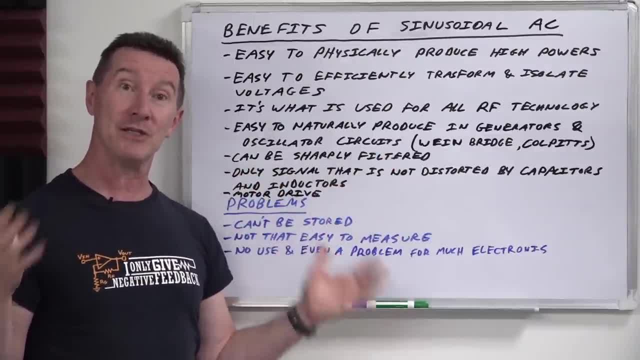 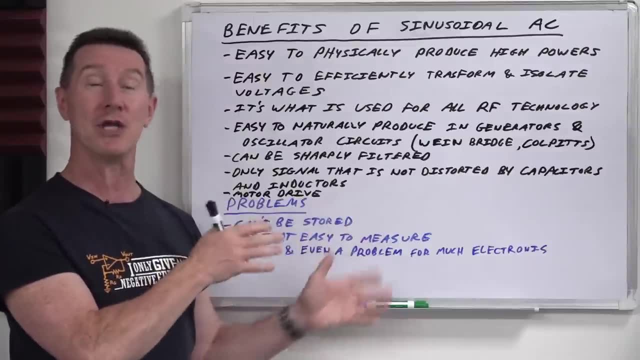 can do with these types of wave forms, and there's a lot of great things, especially when you're using this666. These days. solar is a big thing and it generates DC, but you know, still, the majority is probably going to be coming from some sort of AC generator, be it wind, hydro, coal, nuclear, whatever it is. 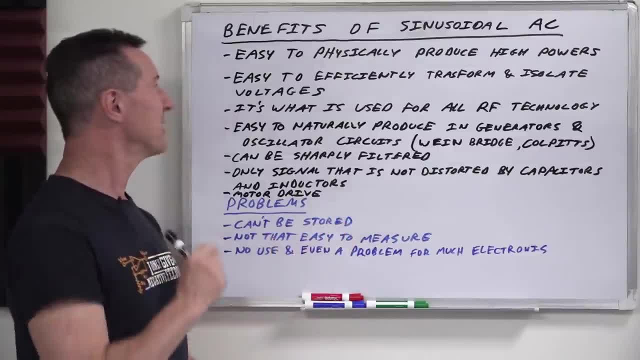 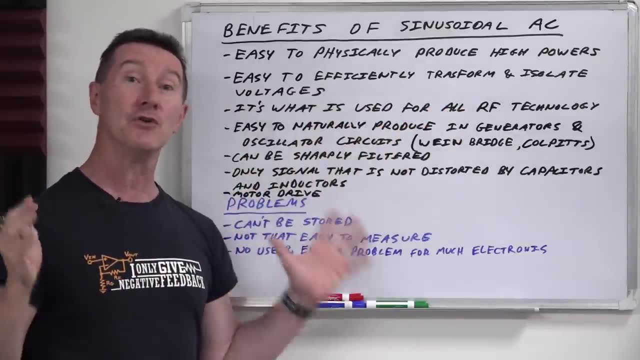 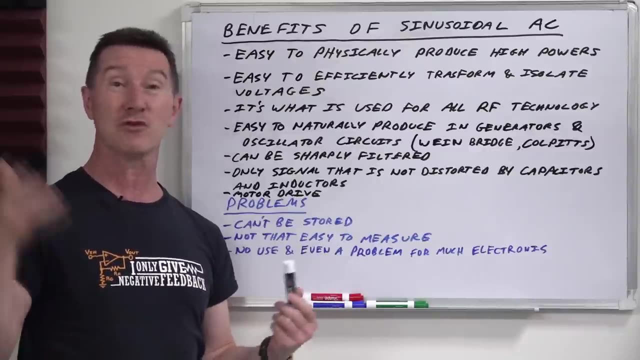 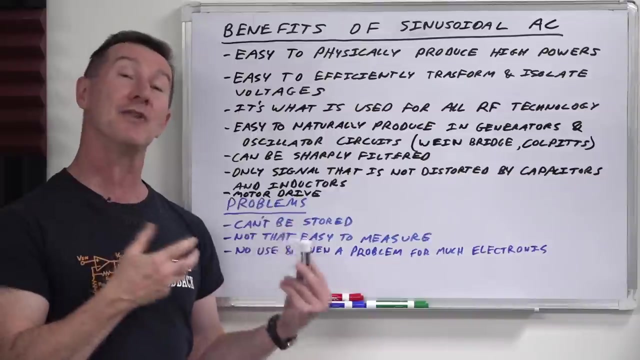 And because the sinusoidal waveform is only one frequency- and I'll talk more about that in a minute- it's easy to efficiently transform and isolate these voltages using transformers. So you go from like 500,000 volts, 500 kilovolts or even 700 kilovolts, I think. these days AC transmission lines, those huge ones, they're easy to step down and you can do that very efficiently using AC, sinusoidal AC in transformers. 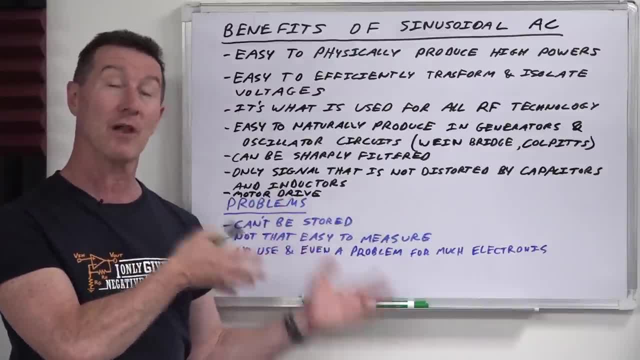 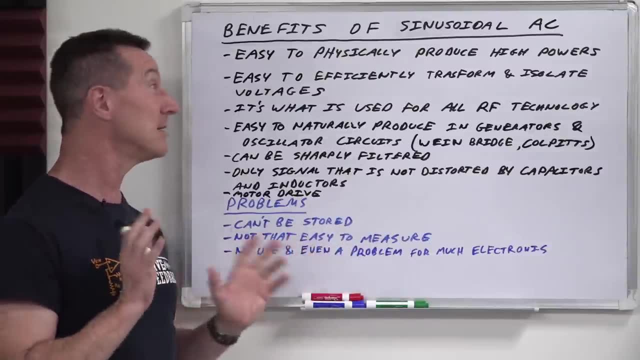 They're incredibly efficient and you can use those at the signal level as well if you're designing circuits. audio and other telecommunications type stuff can be isolated using transformers. Easy peasy, Because a transformer is just a coil of wire and like a piece of ferrite. 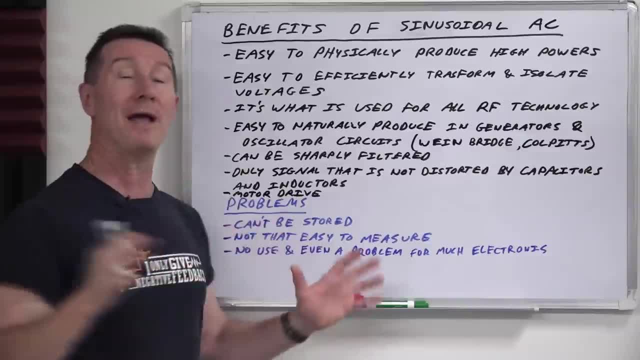 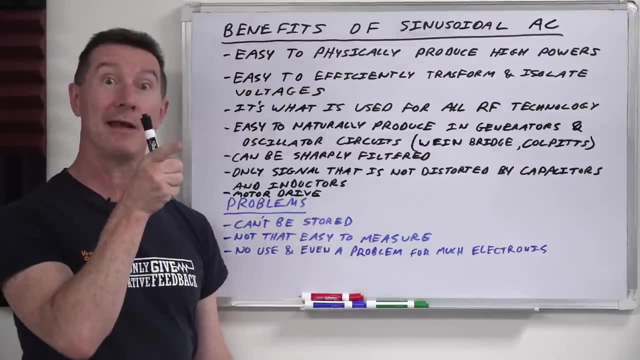 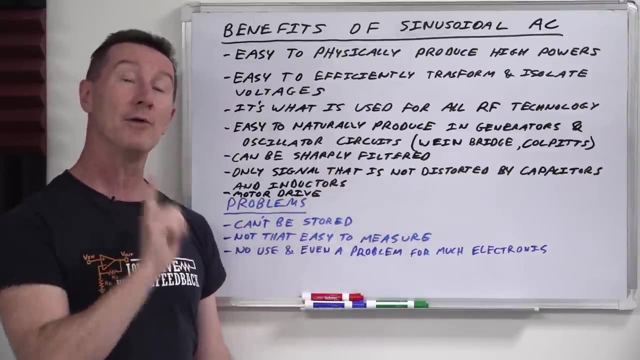 It's really simple stuff And it's what's used for all. basically all RF and communications technology is basically you can't just put DC on an antenna and have it transmit something. It's got to oscillate, And if it oscillates using a sine wave, that is one pure frequency. 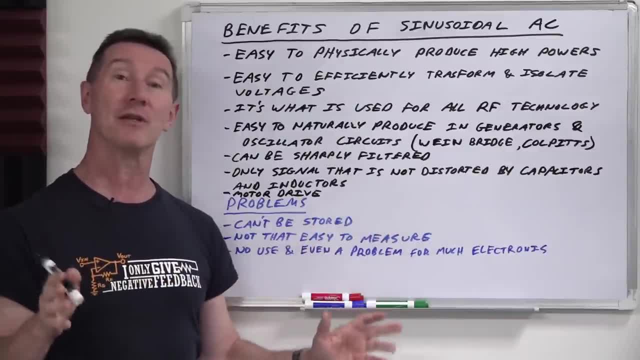 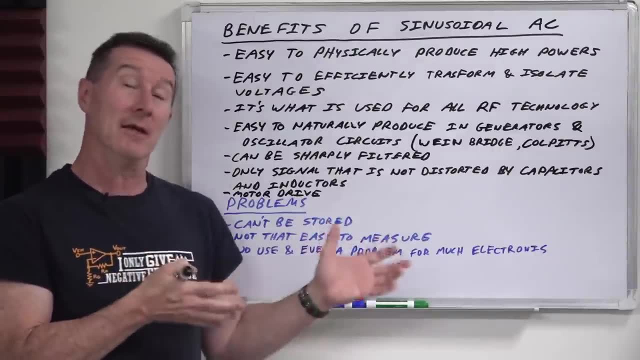 Because don't want to go into it in this video, but you've probably heard me mention Fourier before And Fourier's theorem, or theorem Fourier transforms, as you've heard about FFTs in, basically, oscilloscopes. this is how, like, a spectrum analyzer works in your oscilloscope: Fourier transforms. 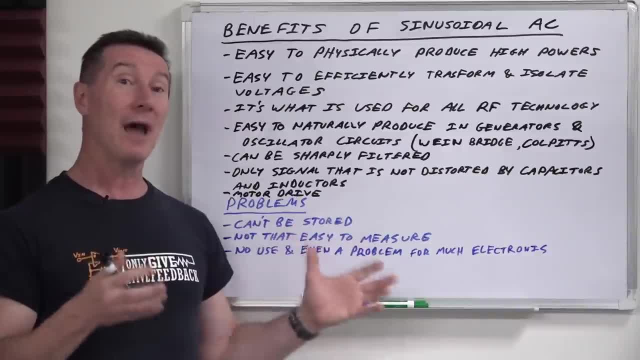 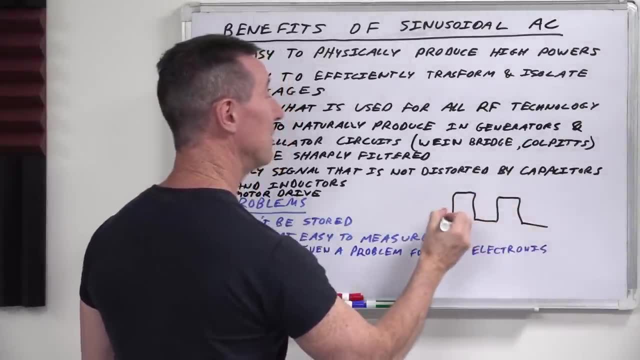 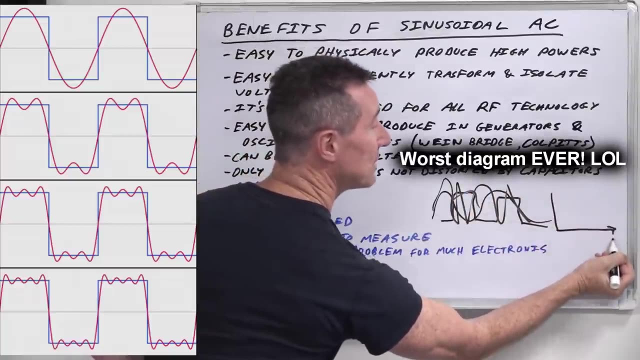 Fourier theorem basically says that any wave shape at all is made up of sine waves. So if you've got a square wave like this, it's actually made up of sine waves at lots of different frequencies. So when you plot a frequency spectrum instead of time, that's F. 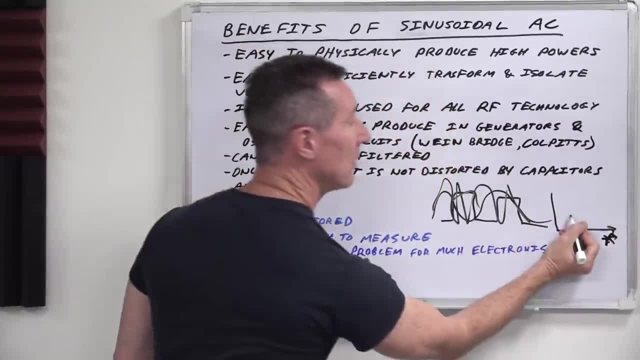 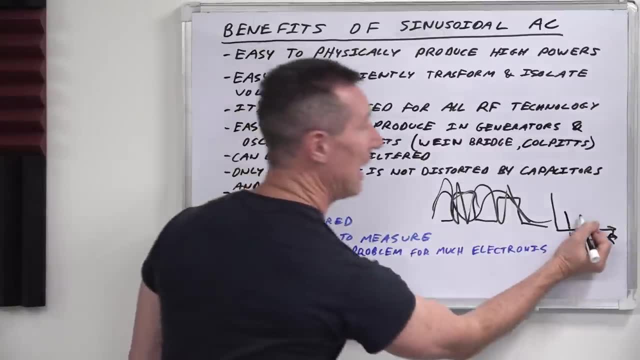 That's simple. It's supposed to be F there. trust me, Frequency like this: if you've got a sine wave, it's just one line on your spectrum analyzer Say that's one kilohertz or something like that, And then you might have another line here at harmonic multiples of that, things like that. 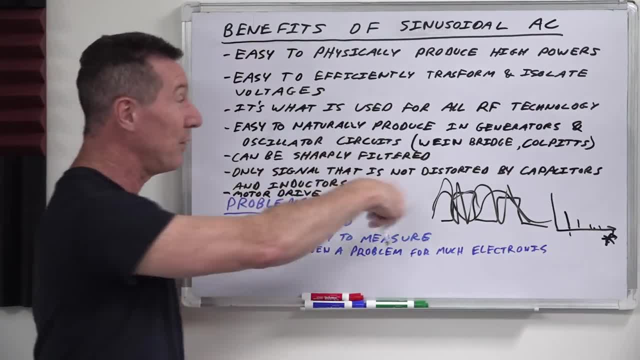 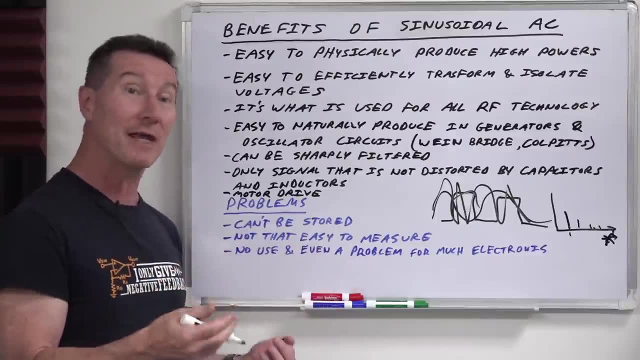 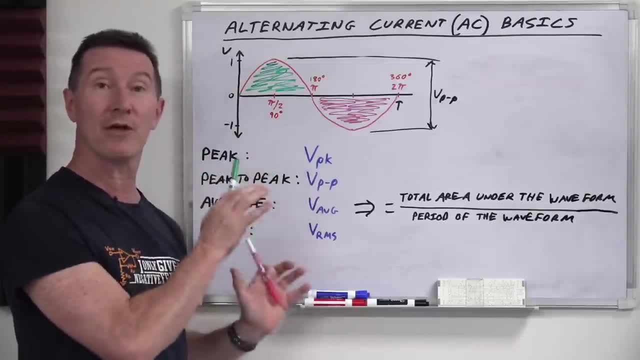 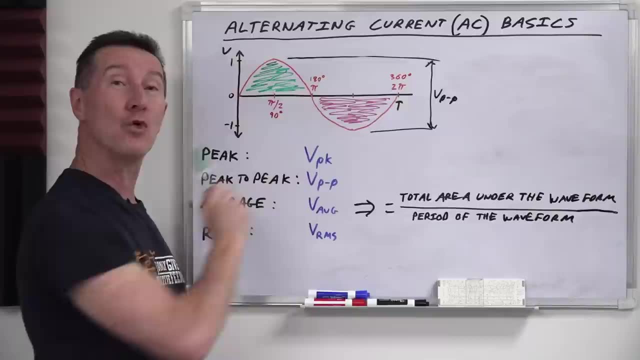 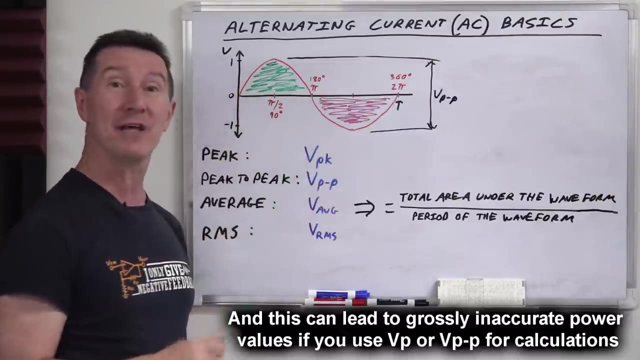 Now one of the downsides about peak and peak-to-peak voltages: while they're very commonly used, they don't actually tell you anything, any information at all about the actual waveform shape. It doesn't actually care. This could be a perfect sine wave, could be a triangle wave, a square wave, doesn't matter. 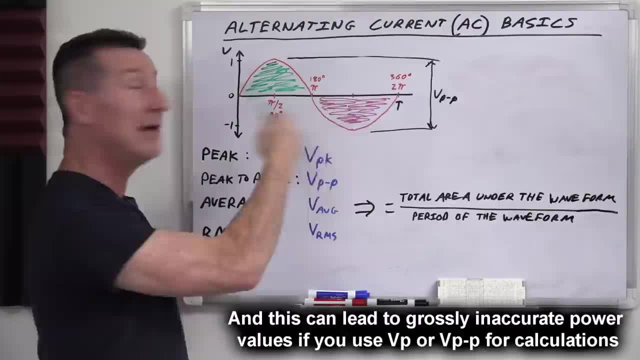 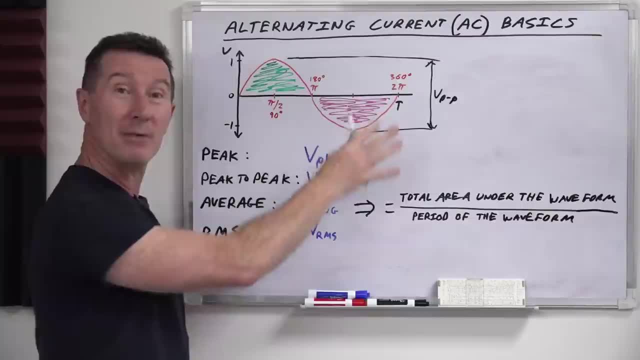 What this waveform is. if it goes to plus one up here and minus one down here, it doesn't matter. It could have a tiny little spike like this tiny little spike down here. It could be like a. you know, that could be a very poor power factor, as we've looked at. 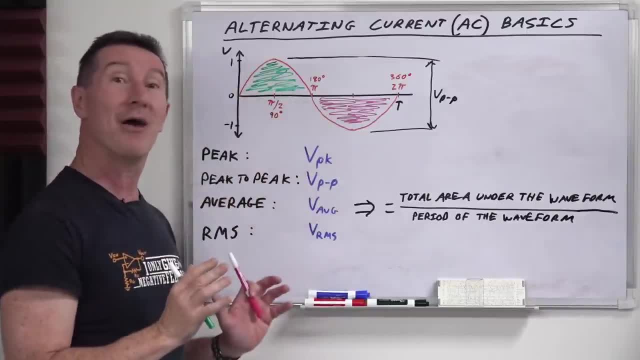 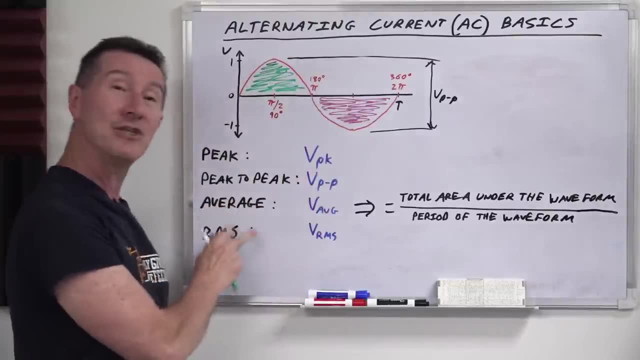 mains waveform or something, The peak-to-peak. it doesn't matter what the waveform is, The peak-to-peak is just the actual instantaneous peak value, like that. But average and RMS they're different. They actually take into account the actual waveform itself. 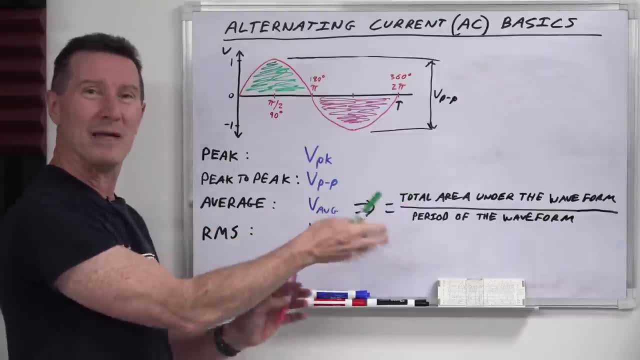 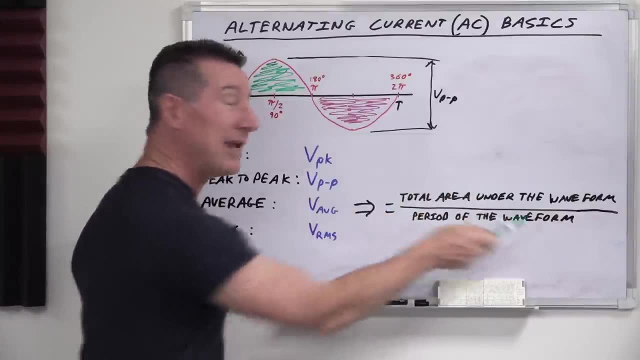 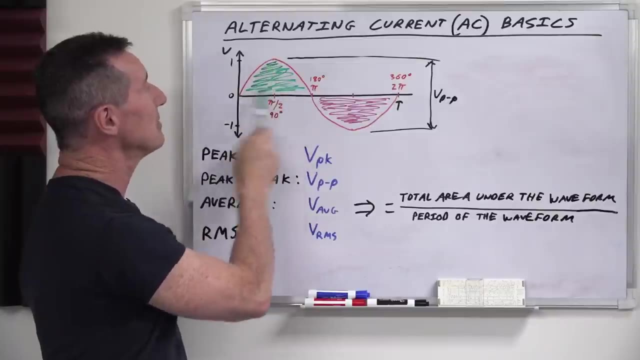 Now, the average value is defined as this, and there's several different ways to sort of explain it, but this is the way I'll do it. It's the total area under the waveform Divided by the period of the waveform. So the total area under the waveform, that means all this area under here, like this: 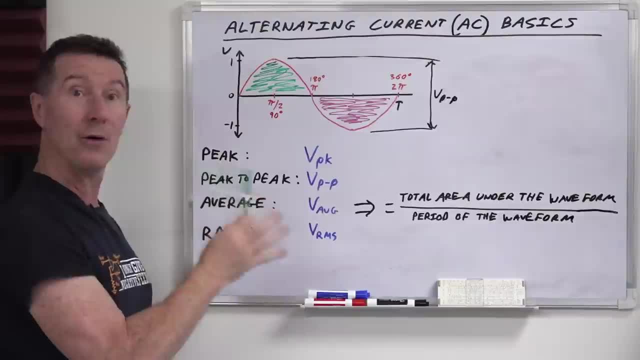 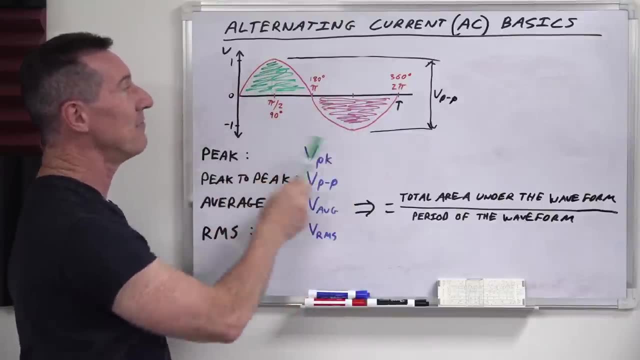 like to the axes. you've got to have it like to a reference axis, So all the area under there. but we've also got all this area under here And this one's positive and this one's negative and because it's a perfect sinusoidal waveform. 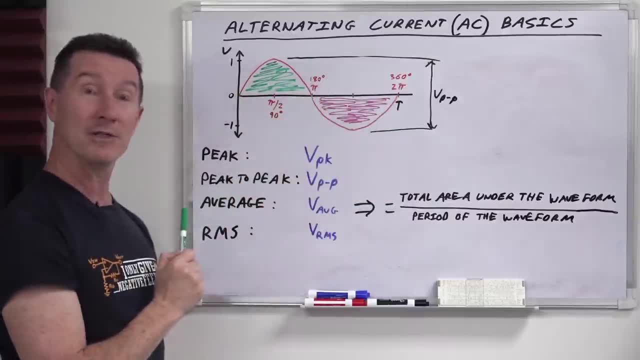 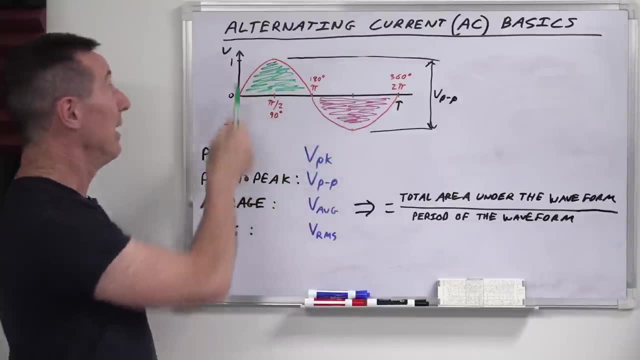 or it could be a perfect square wave, for example. it doesn't actually matter If the area above the axis here is equal to the area below the axis here and they're both the same amplitude. like this, the average value will actually come out at zero. So if you feed an AC voltage, a perfect AC voltage with no DC offset, into your DC multimeter, which reads average value, it'll read zero. And also for multimeters that aren't true RMS, multimeters that'll have true RMS. 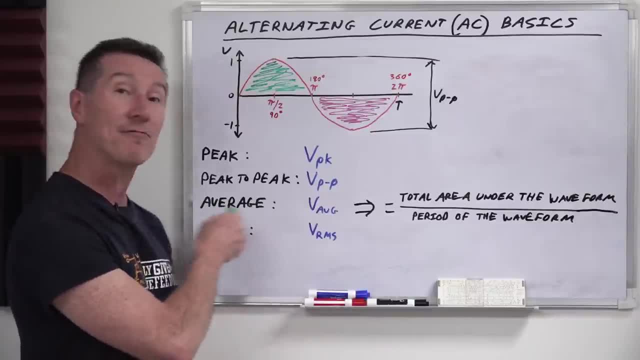 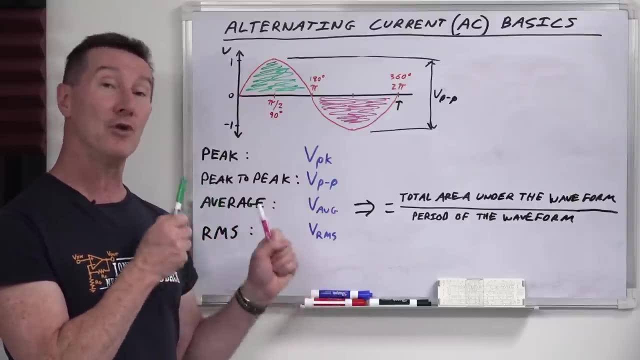 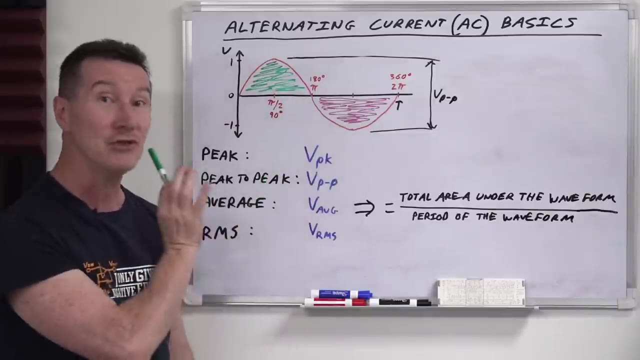 are written on them. usually they will actually be what's called an average responding multimeter for AC. So what that means is that it assumes that the waveform that you're measuring in AC voltage mode or AC current mode on your multimeter is a perfect sine wave. If it's not a perfect, 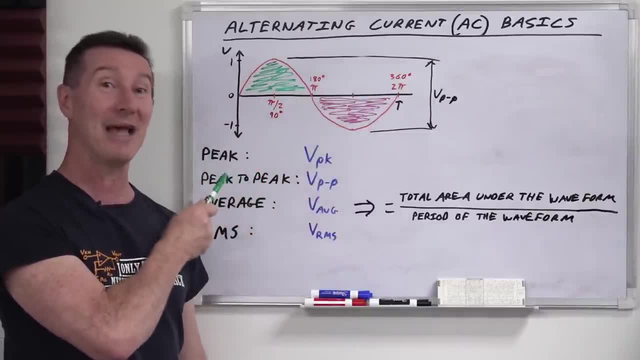 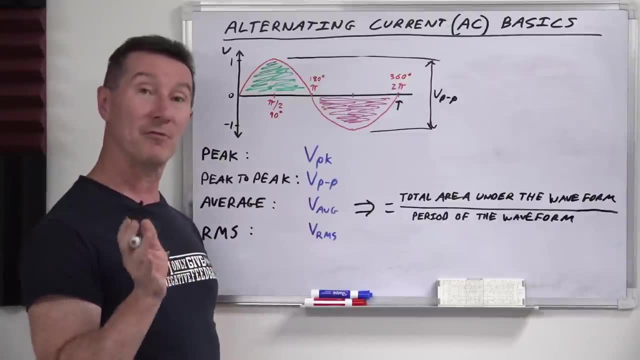 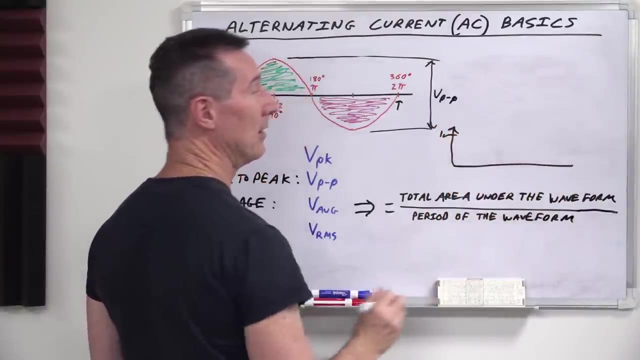 sine wave, it's going to give you an error. It's not going to be accurate because the multimeter has only been calibrated to assume a perfect sine wave. To give you another example from digital electronics you might be familiar with if you've got a V here. so that goes up to one. 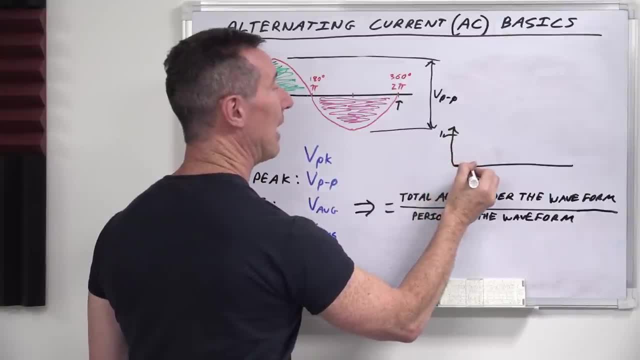 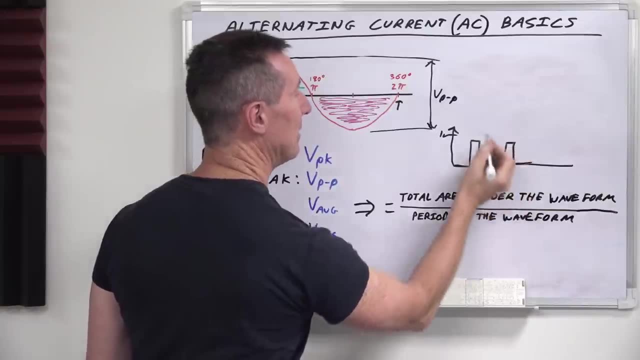 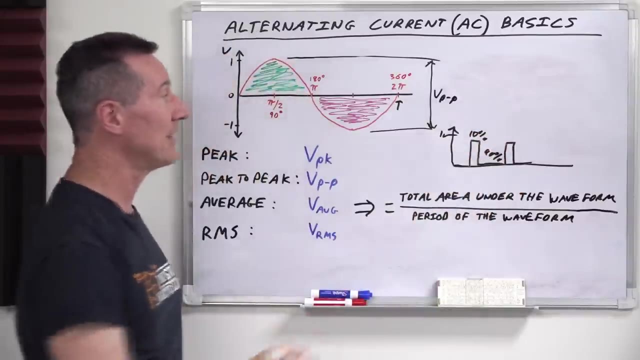 volt there. this is time. and if you've got a pulse width modulated square wave that is like this, let's say that this is 10% of the time and it's 0, 90% of the time, like this: 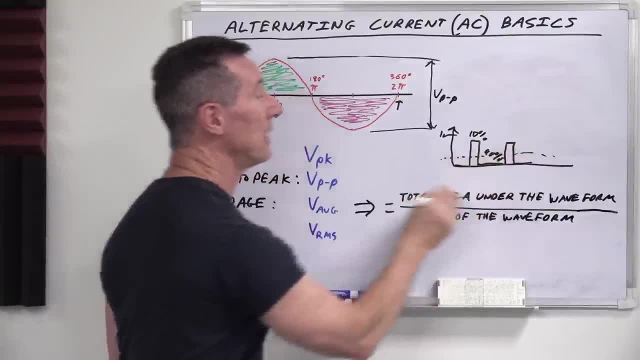 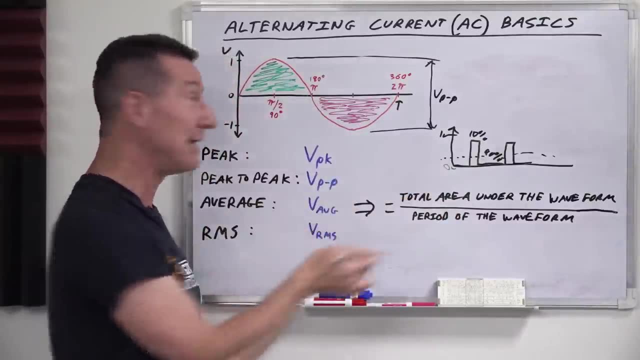 what is the average value going to be? Well, our axis is 0, it's going to be 0 volts down here, like this: everything's above the axis. it's not actually an AC waveform, it doesn't go negative, but this can actually apply to it. doesn't matter where the 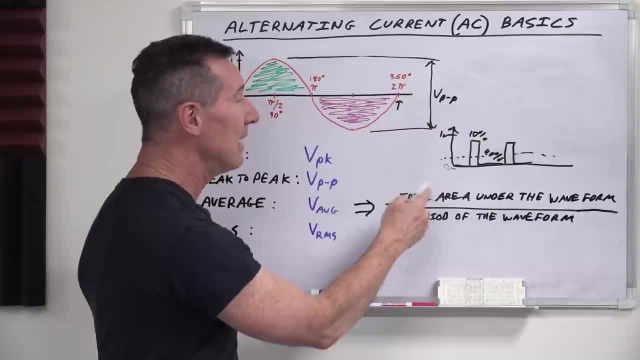 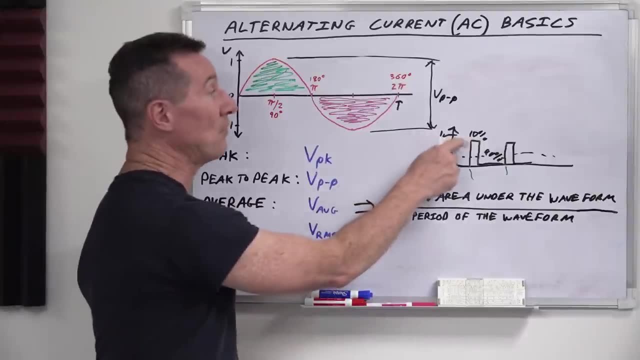 reference point is. our reference point in this case is 0,. okay, the total area under the waveform. so the period from here to here it'll be 1 volt for 10% of the time, multiplied by 0 volts for 95%. 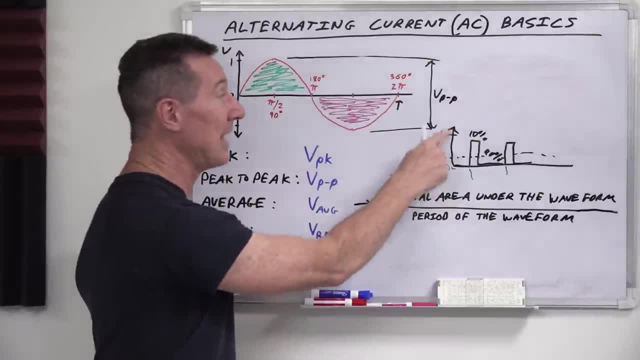 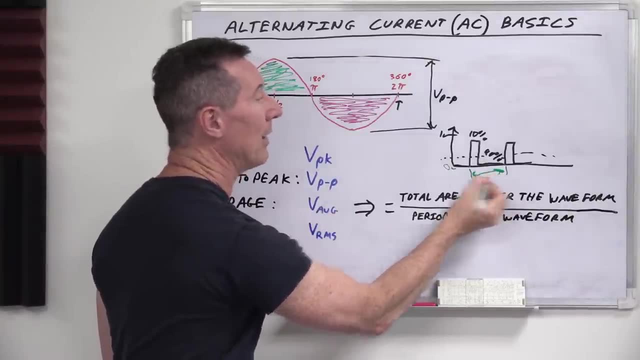 of the time. so therefore it'll actually equal one tenth of that, or one tenth of that. 0.1 volts will be your average value over the period of one waveform. So let's analyze a half wave rectified sine wave, and you'll be familiar with this if you've done. 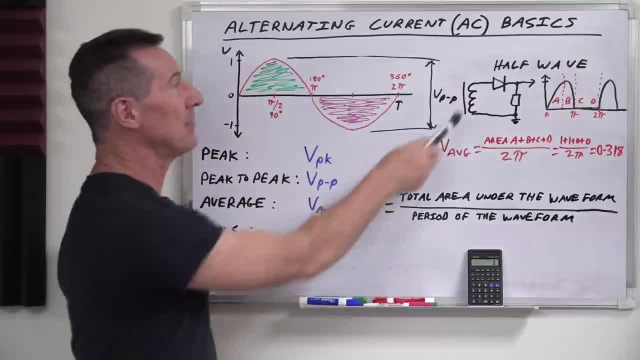 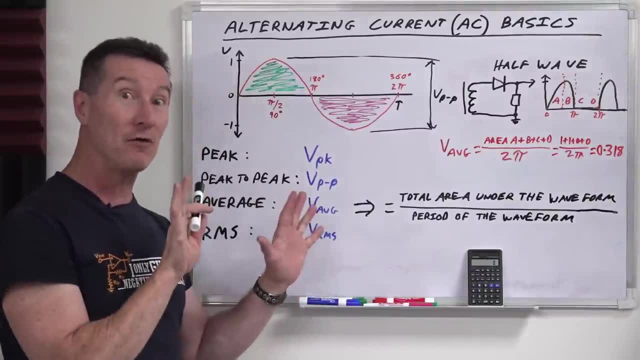 made any do-it-yourself basic power supply from a transformer. so this is our AC transformer. just got a single diode in there. it's just driving a load. there's no filter capacitor, because that smooths it out and ruins your day. so we've got a waveform that looks like this: 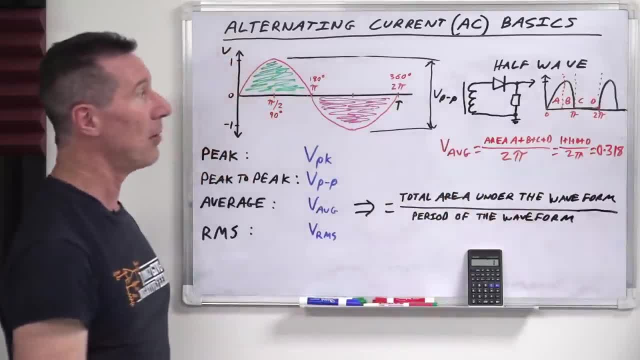 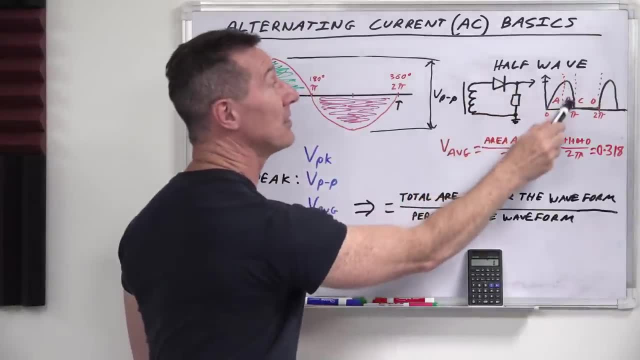 it's, here's our total period here, from 0 to 2 pi or 0 to 360 degrees, and it's, as its name suggests, is a half wave rectifier. it only rectifies the positive half, The other half of the waveform down here, when it goes negative. 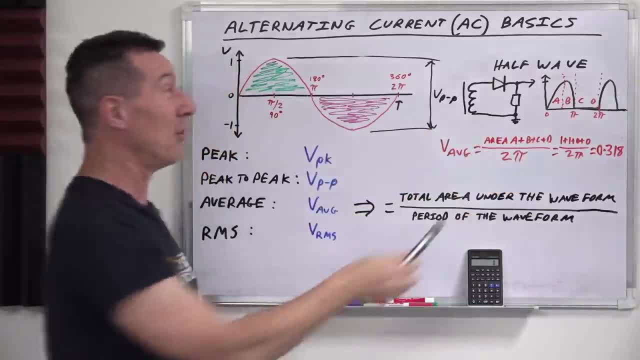 the diode is reverse biased, so it doesn't conduct at all. so you just get 0, so you get this half wave rectified waveform. Now we'll analyze this waveform using our formula here, and there's several different ways to look at it. but because it's a sine wave, what I'm going to do is like this half. 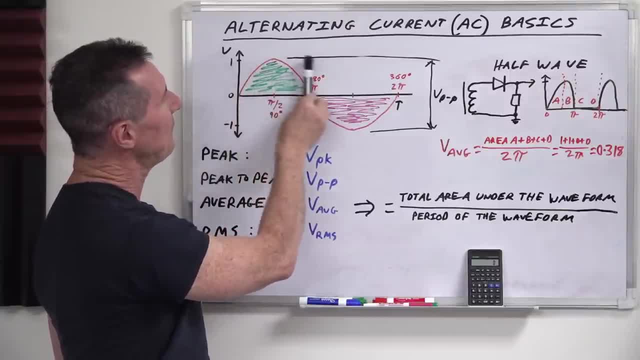 of the sine wave from 0 to 2 pi or 0 to 360 degrees, and it's as its name suggests is a half wave rectifier. so what I'm going to do is just split it into quadrants like this, so just assume that there's like 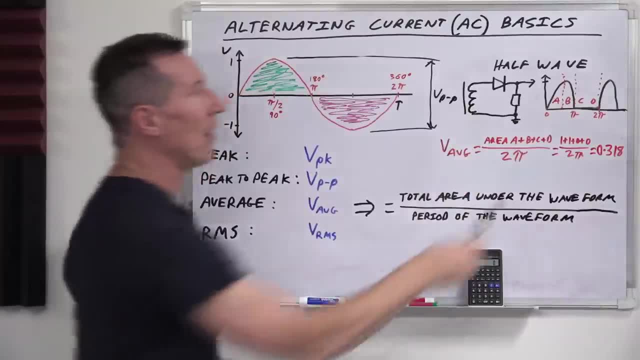 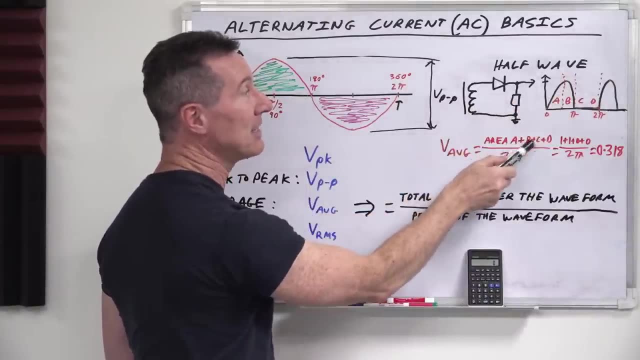 four different areas that we're calculating here for our one waveform, from 0 to 2 pi. so it's the area of A here, plus the area of B, plus the area of C, plus the area of D. you remember, it's the. 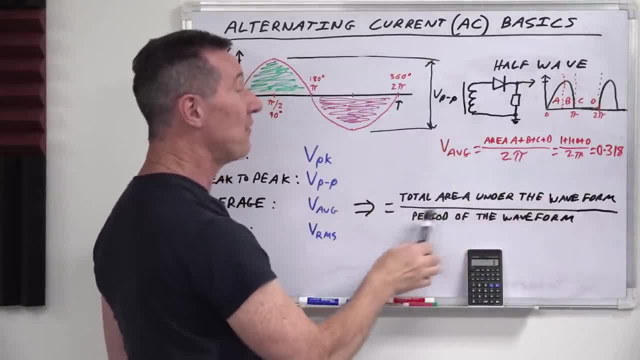 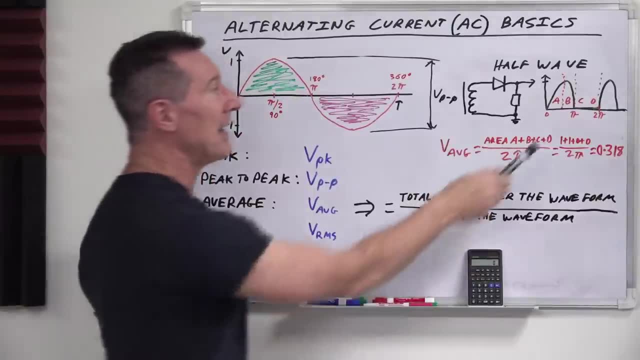 total area under the waveform divided by the period of the waveform, which is 2 pi. so area A plus B plus C plus D divided by 2 pi. Now we'll just normalize the area to 1, we'll just call it 1,. 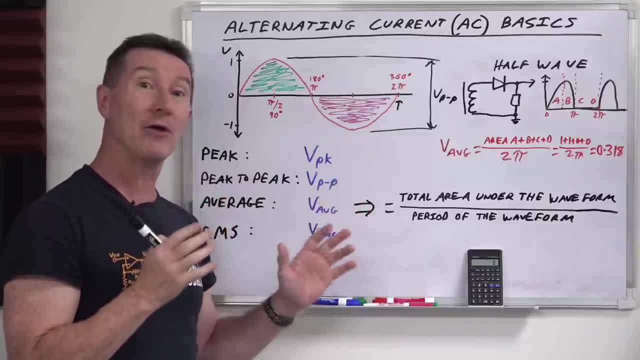 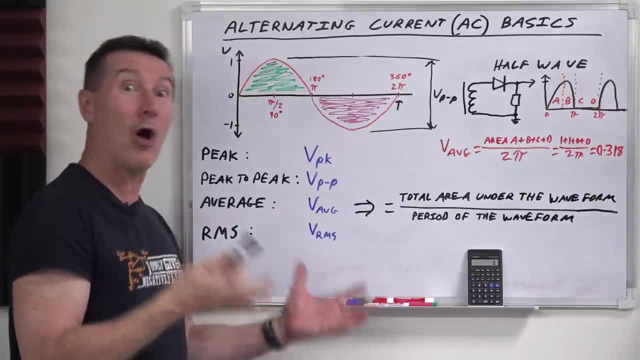 because we're not talking about any actual absolute value here, so we'll just normalize it to say that area A is 1, or area B is identical to area A. obviously it's a perfect sine wave. so 1 plus 1,. 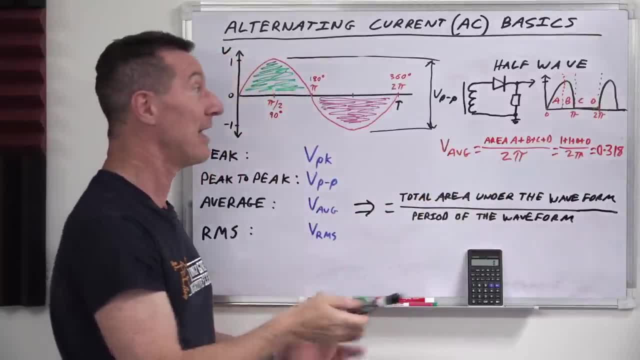 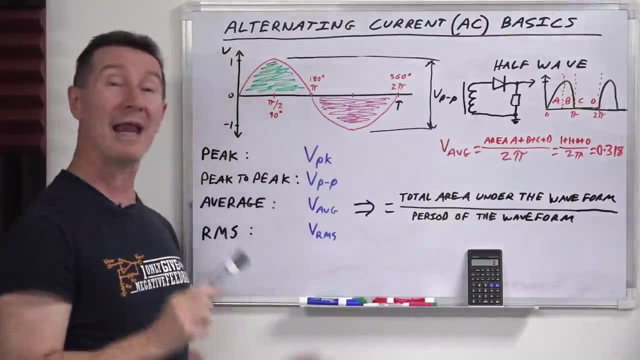 and then area C and D are of course 0, there's nothing there, so it's 1 plus 1 plus 0 plus 0, or 2 divided by 2 pi, And then we'll come up to say: 3 pi equals 2 pi first, so that 2 pi is equal to 0.318, not 0.318. 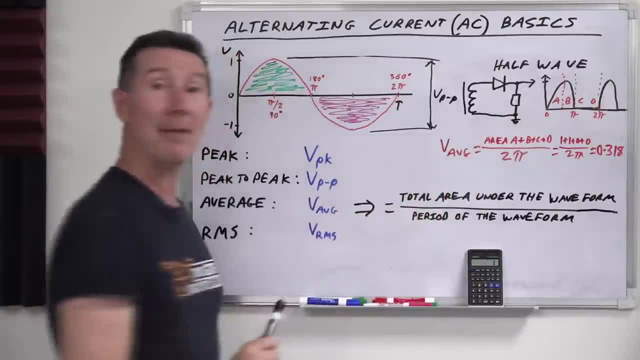 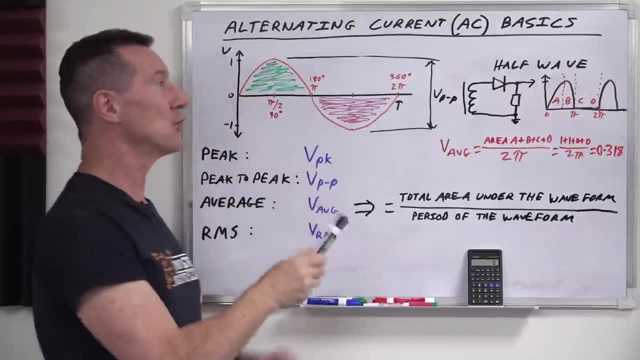 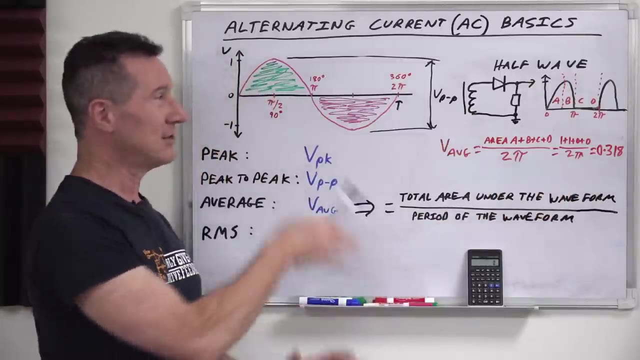 volts. 0.318 is the factor that you then multiply by your peak value up here. but that is just a factor that you multiply by the peak value up here to give you your actual average voltage for a wave, rectified waveform, And that's a common number. 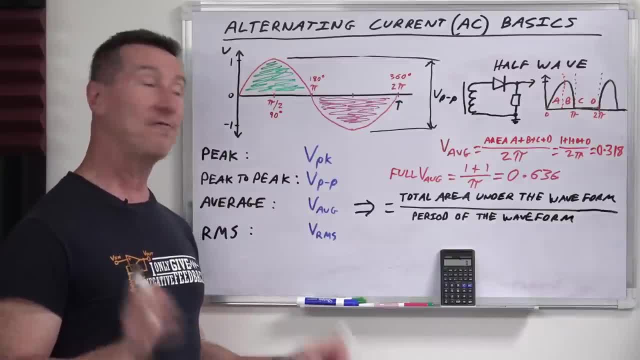 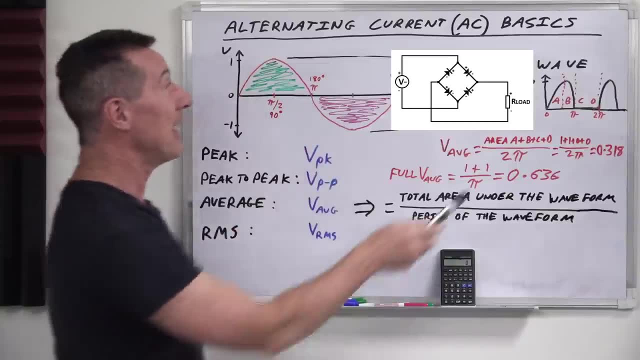 number you go: oh yeah, that's half wave And we'll now look at a full wave. bridge rectifier. I haven't bothered to draw it, but basically, if you're familiar with them, I'll put up the circuit here. Here it is Now. this will give us a waveform that then looks now like this. So we'll 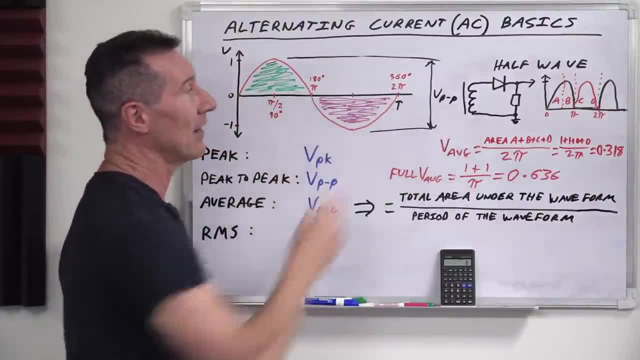 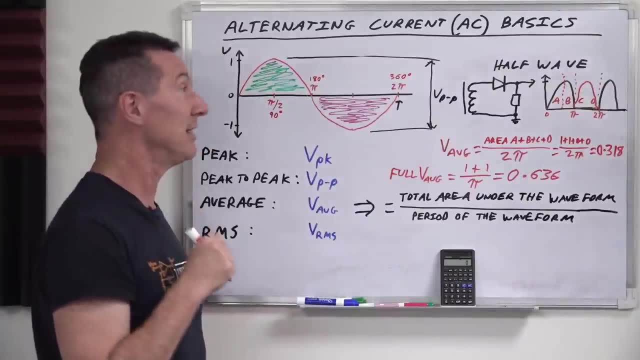 get two humps, because it does the positive and the negative cycle as well. But because that's now identical and we've doubled our frequency, say it's 50 hertz here in Australia, not any of that 60 hertz Yankee rubbish. if it's 50 hertz then it actually becomes 100 hertz now because 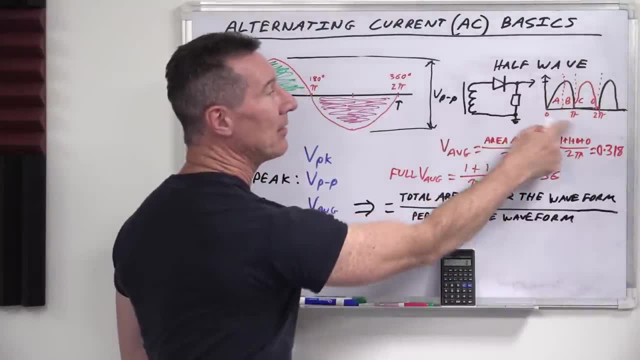 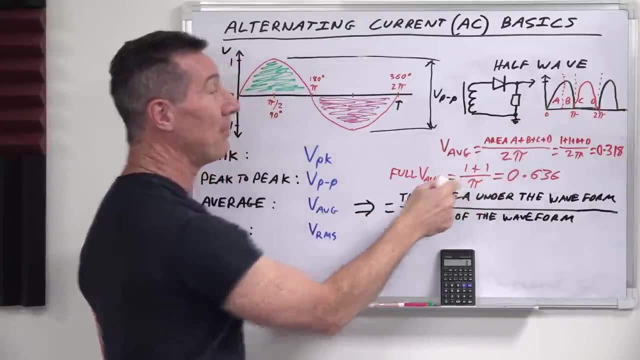 the waveform is repeated, So our period is not 2 pi anymore, it's just pi, like this: So it's 1 plus 1, area of A plus area of B, divided by pi, which is 0.636.. Wait, wait, no, isn't that meant? 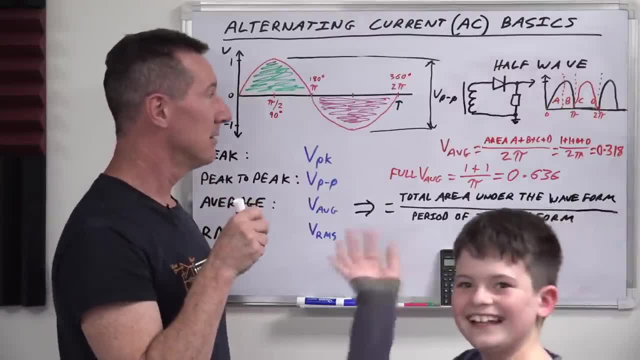 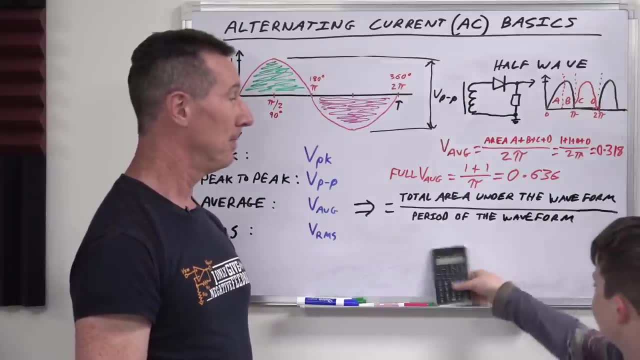 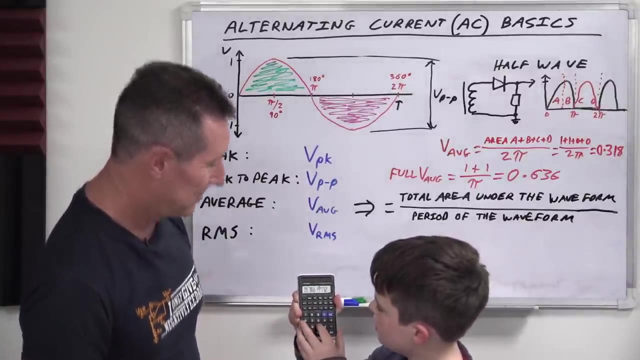 to be 637?. Here's Sagan: 637.. Yeah, Why? Why would it be 637? Because when you go into the calculator here, if you go, 2 divided by pi Equals, Equals, 0.6366.. 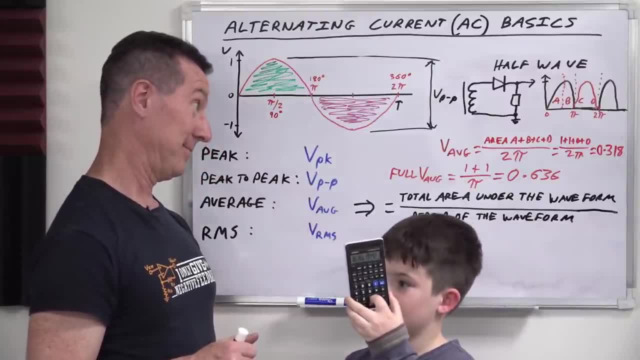 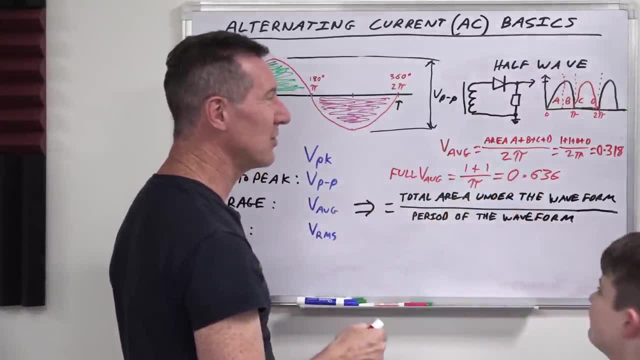 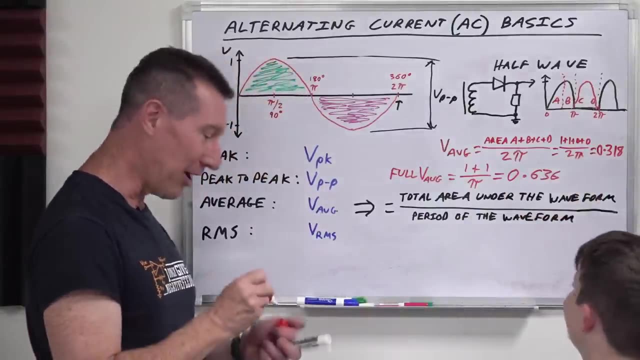 So you reckon, Round it up to 0.637.. 7.. Well, I'm going to say that it's 636, because that's kind of like symmetrical, and it's double 0.318. that I rounded It was 0.318 and we measured it before. So I'm sticking with 636, you reckon 637?? 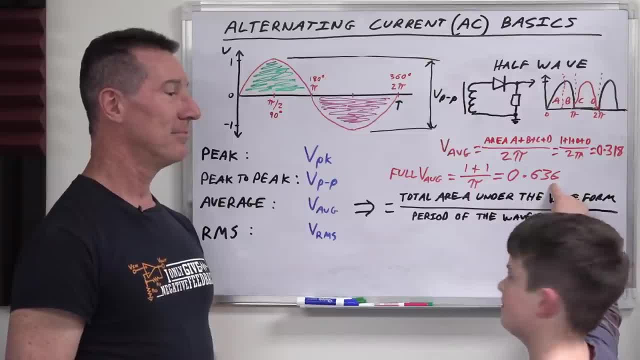 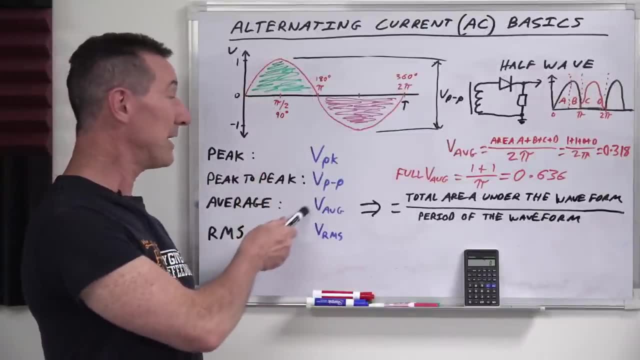 I'm the type of person who likes symmetrical and all but 637.. OK, leave it in the comments down below. Thanks, Sagan. Yeah, Now the thing about peak, peak to peak and average voltages is that they're absent. 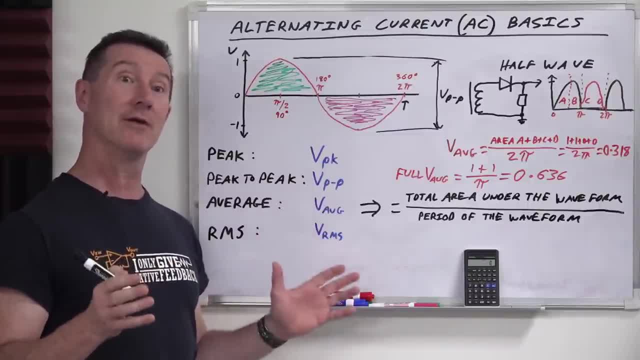 and currents is they're useless for measuring power. You'll get the wrong value. In fact, you'll get zero Cause. let's just assume that this is a current waveform. OK, this is a current waveform and this is a voltage. 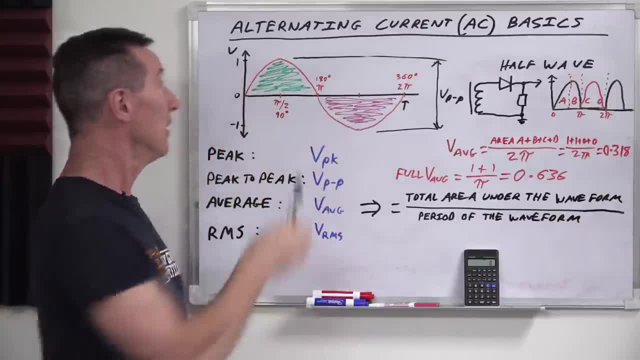 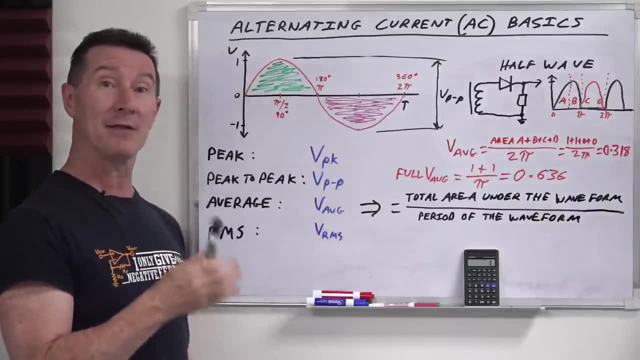 Okay, and you've got it: dissipating power into a resistor. There's going to be power dissipated in the resistor on the positive half. like this, There's going to be power dissipated in the resistor on the negative part of this, because power doesn't care whether the voltage is positive or negative. 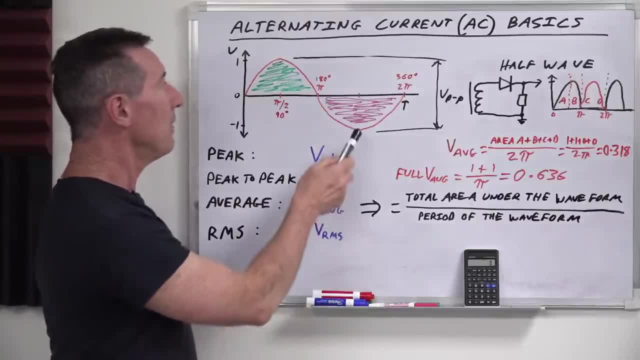 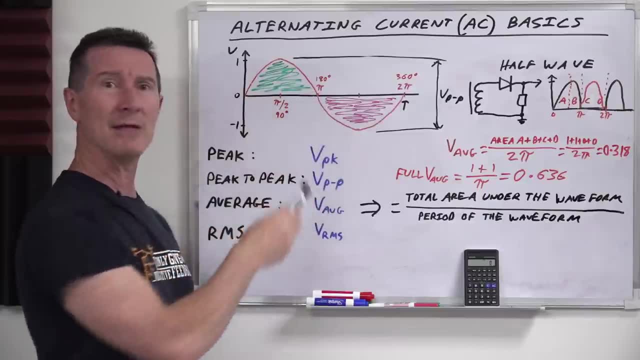 It's just the power dissipated in the resistor or the load, Then well you're. but if you measure the average current, the average current is going to be zero and zero times p is i squared r zero. squared times r is zero. 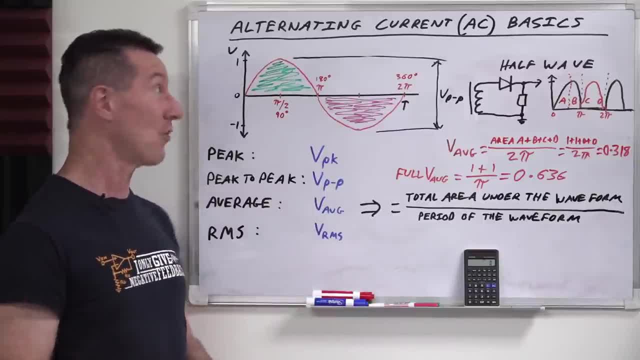 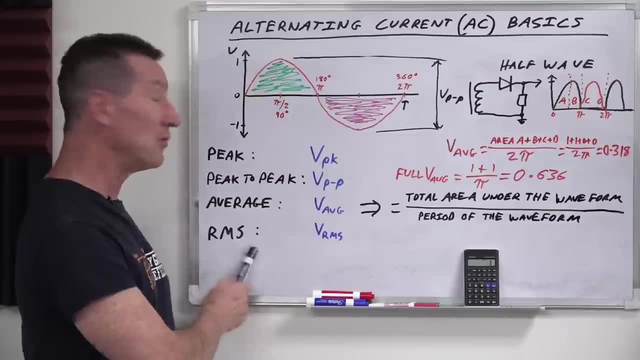 So you've got zero power dissipation. Uh-uh, Go, try it. Put an AC waveform into a resistor. You're going to dissipate power. So it doesn't work. In this particular case we have to use RMS. So RMS stands for it's right in the name, the root mean squared. 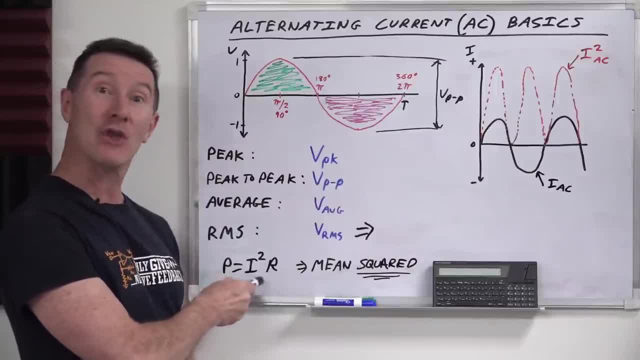 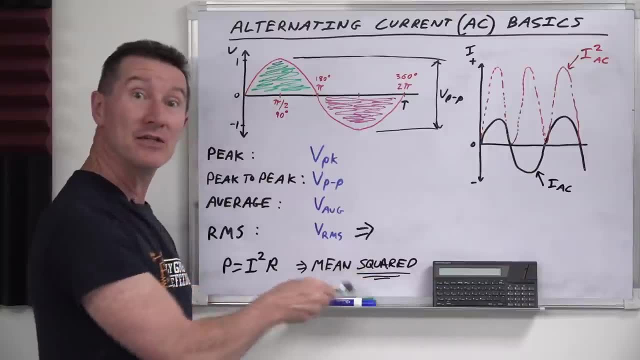 Where does the squared bit come from? Well, power equals. i squared r, There's a squared factor in there and when you square that, that is the mean squared. So if we have a look at the waveform over here for current, we've got our regular AC current waveform. 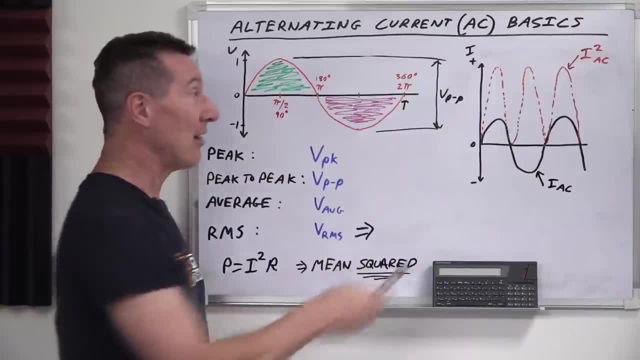 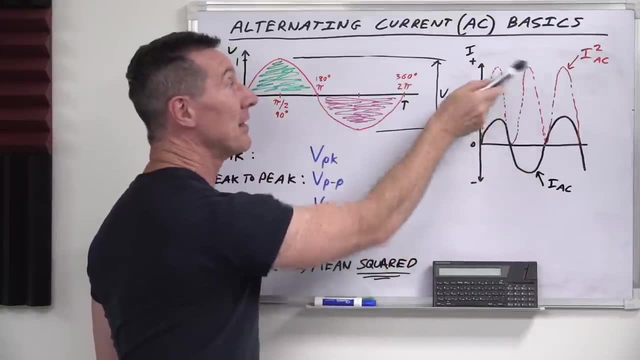 We'll call that IAC here. Then if we square that current, we square it like: take every single point on this waveform and square it. the number, any negative numbers, they're going to go positive like this. So it's going to be squared. 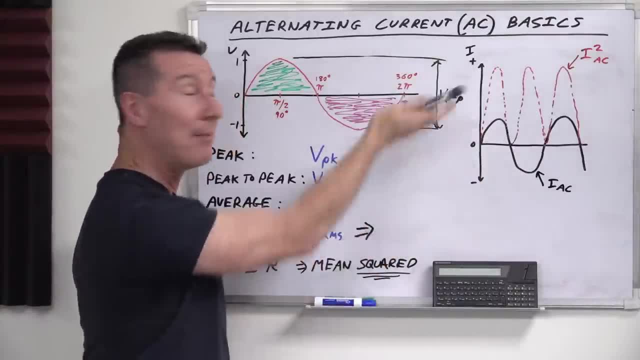 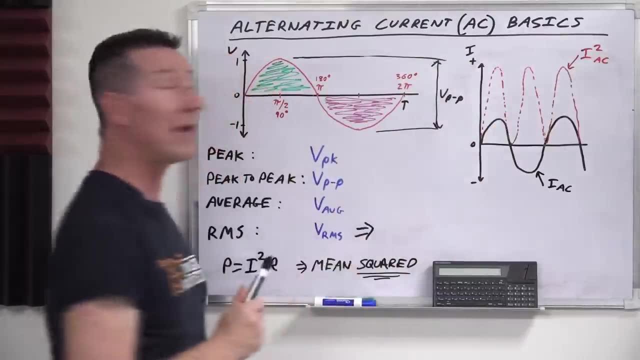 So it's going to be much larger, like this, and it's all going to be shifted up on the positive half of the reference axes Like this. So we'll call that I squared AC. So that's where our squared factor comes from. 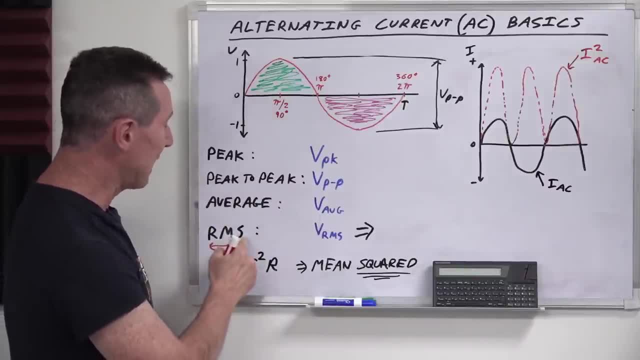 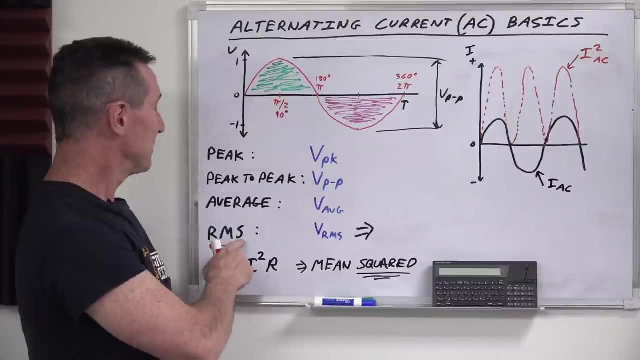 So what you do is you actually work backwards. You take the square first, then you take the mean and then you take the root, the square root. So we've done our squared business. Let's now take the mean. We've looked at the mean before. 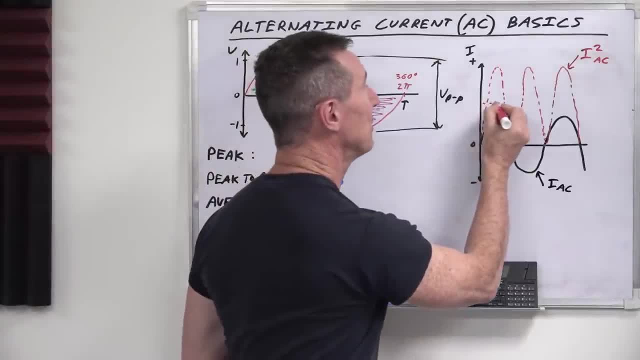 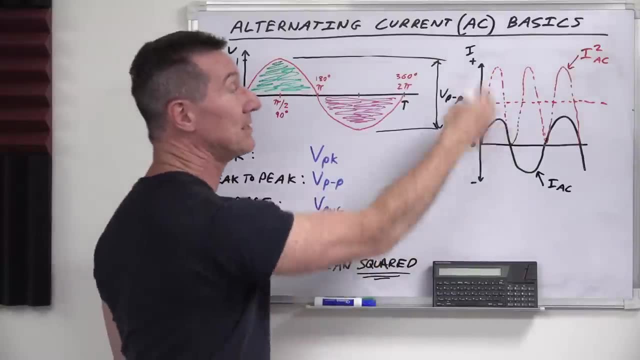 The mean is the average. Okay, it's just another word for average, The mean. then the average is smack in the middle like that, because that's a perfect sign. You saw it on waveforms Squaring. it doesn't change the wave shape. 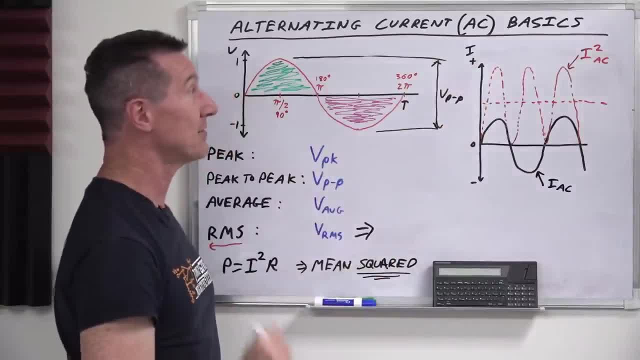 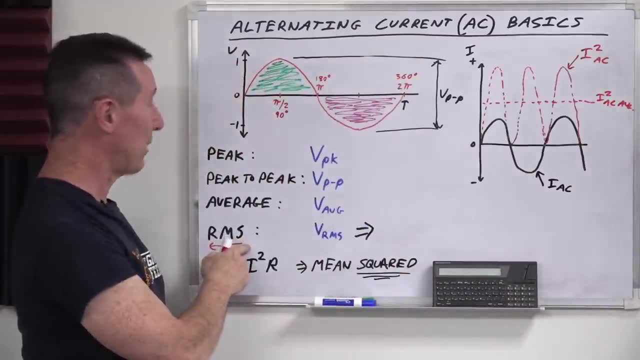 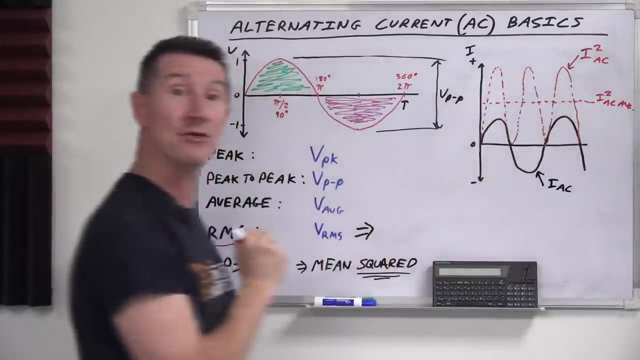 It simply shifts it up and changes the amplitude like this. So we'll call that I squared AC average, like that. That's our average value. So we've done our squaring business. We've done our mean or average business. Now we need to take the square root of that average value. 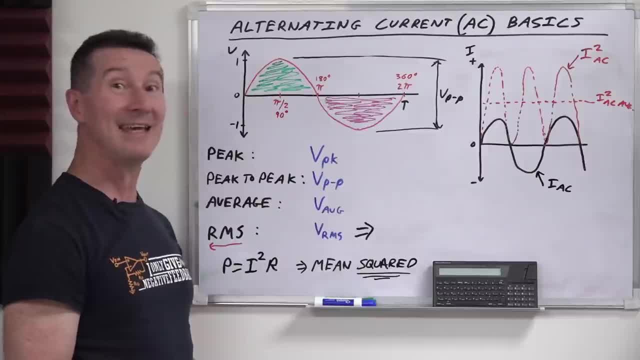 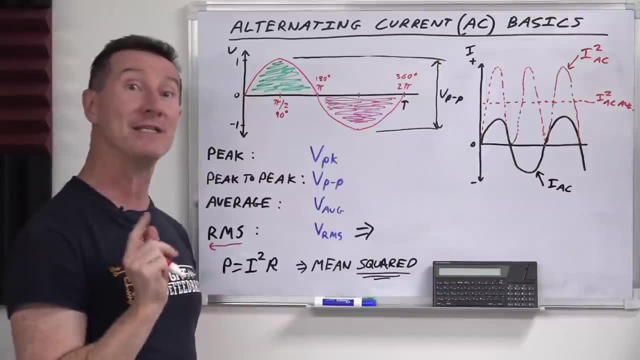 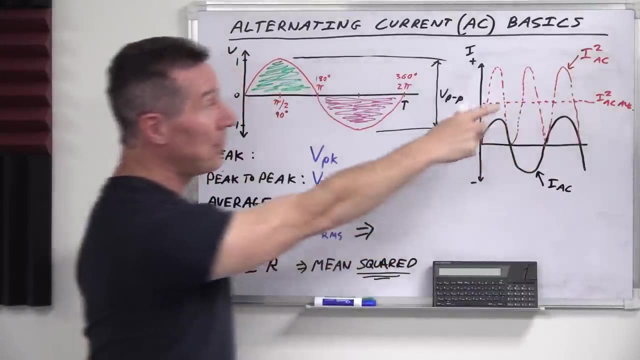 But what is that average value? Well, it's pretty easy. as we looked at before, This is the peak to peak value. Well, it's the peak to peak value of the waveform. It's now the peak value of the waveform I squared AC, is also, I squared, peak. 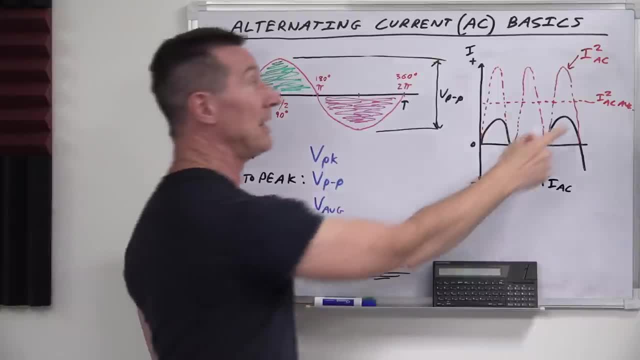 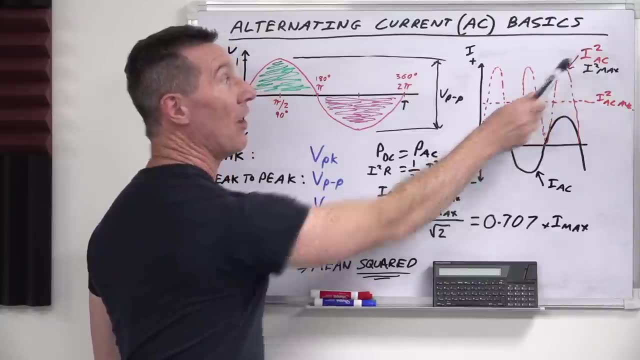 It's the peak value of the waveform, And the mean value is gonna be the peak divided by two. It's smack in the middle, simple. So this is I squared max, as we'll call it over here. Now let's actually go through and 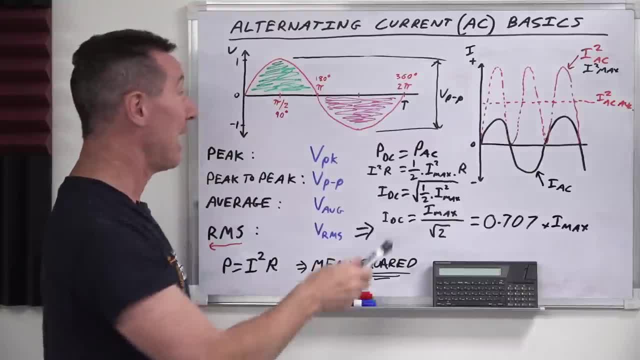 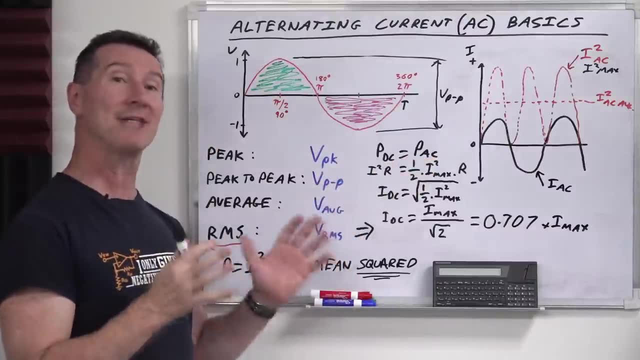 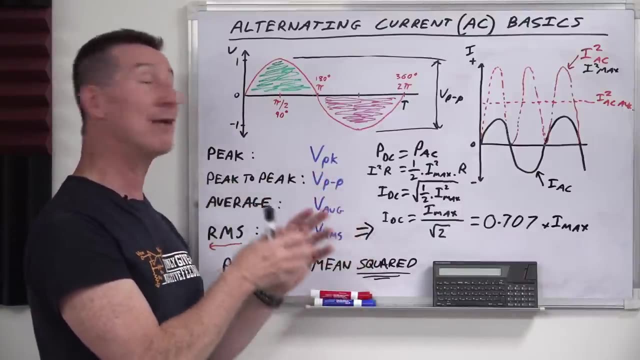 derive the actual answer for our RMS- And you might be familiar- 0.707,. we're getting there Now. the DC power must equal the AC power, cuz that's basically the definition of RMS is that it's the equivalent heating in a resistor for the equivalent value of DC. 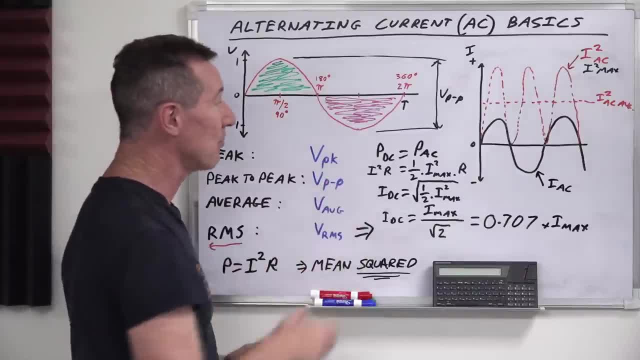 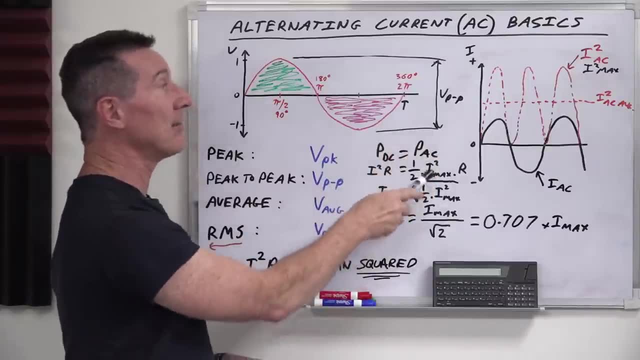 So that's what the RMS value actually is. So how we derive this is well. the power in DC is I squared R- We learned that back at day one- And the power AC here is actually the average value here, now that we've squared it. 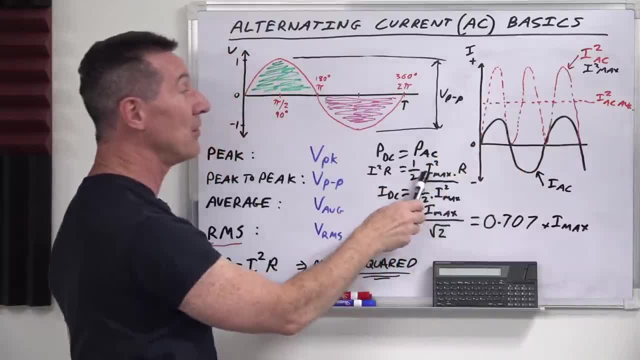 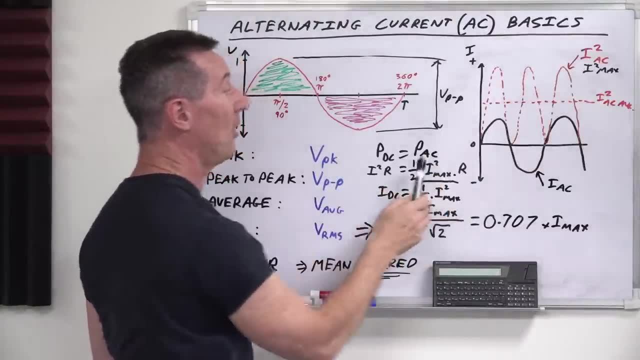 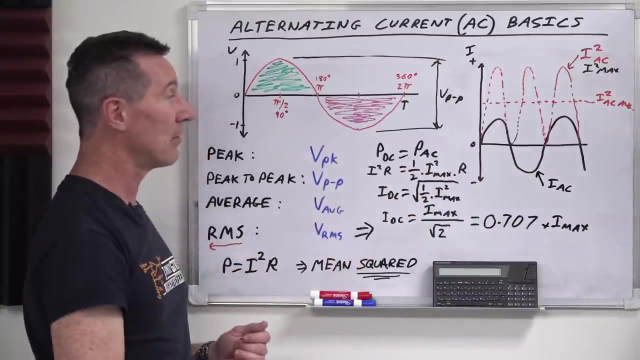 It's no longer zero, it's right up there. It's gonna be the average value times the resistance in the load. So of course that average value is gonna be half of the peak value I max. So you could put average in there like AC average in there, if you want. 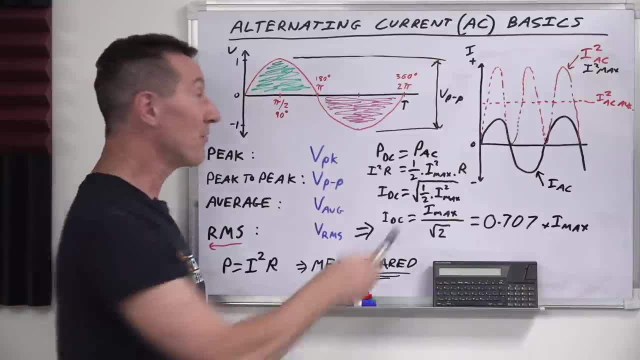 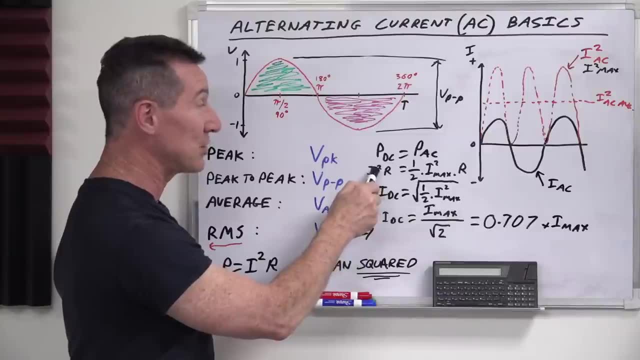 But we'll put half. I squared R max Now because we've got R on both sides of the equations, we can actually take that out And IDC is equal to the square root, cuz we had square here, so we have to bring it over. 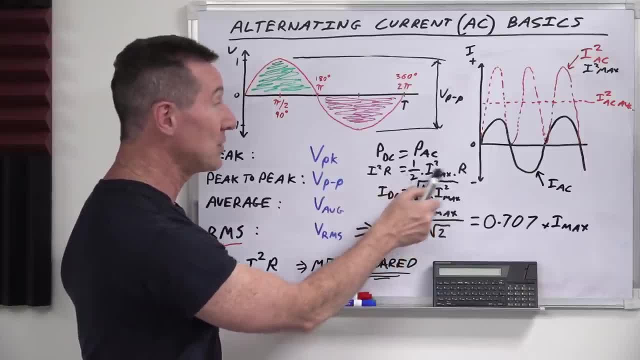 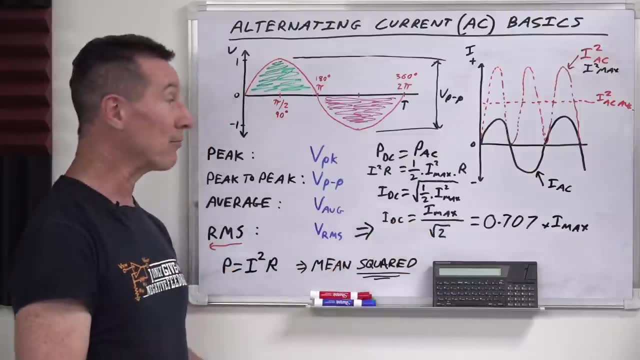 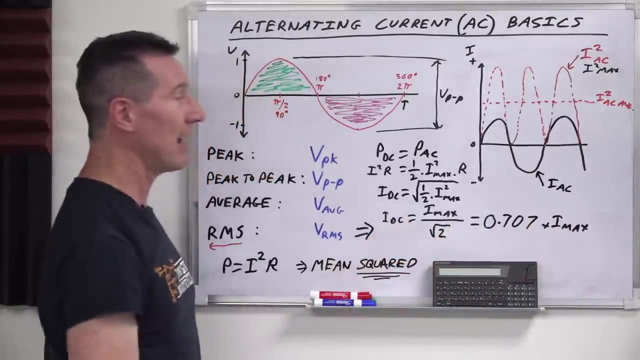 And now it becomes square root, half times that I squared max. And then you can just rearrange that again to be I max on the square root of two. And well, if you say I max is one, then it's 0.707, that's your answer. 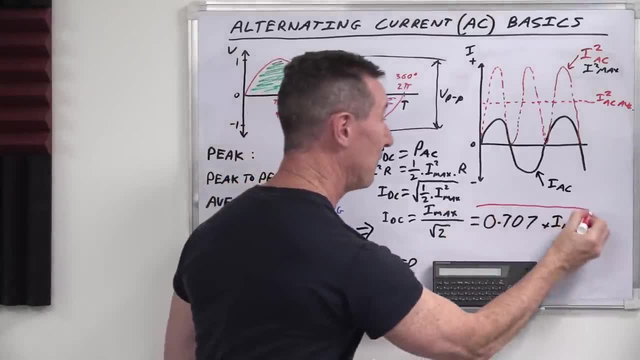 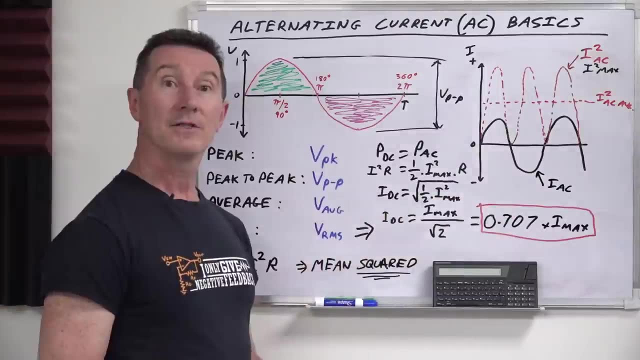 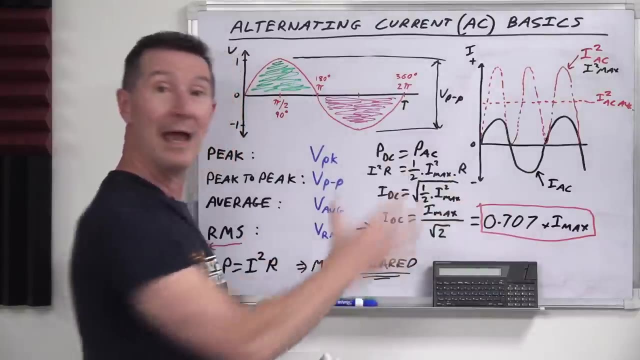 But this is the formula for RMS. Value is 0.707.. 0.707 times the maximum current there. So any time you see 0.707 in electronics you know you're talking about one on square root of two And it's basically RMS. 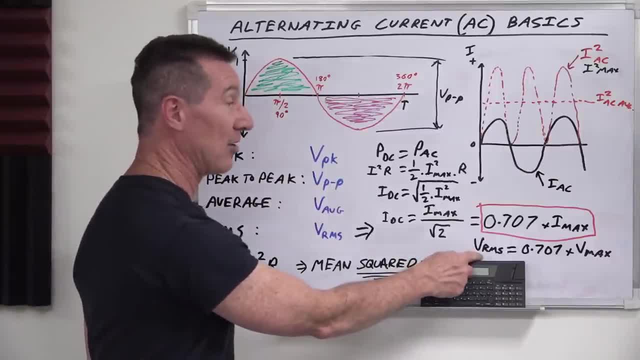 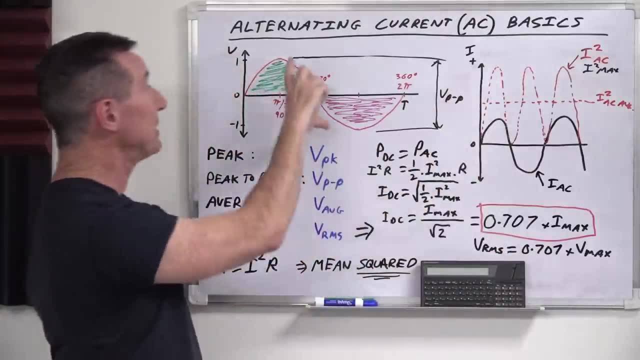 And this also applies to voltage as well. So V RMS, the RMS voltage, is equal to 0.707 times V max, which is actually V peak to peak. So the equation that you have to remember is: volts RMS equals 0.707 times V max. 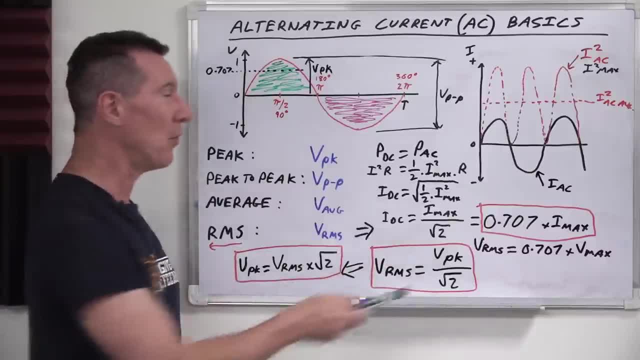 So the equation that you have to remember is volts. RMS equals 0.707 times V max, which is actually V peak to peak, which is actually V peak to peak, Divided by the square root of two. Or you can remember the 0.707 if you want. 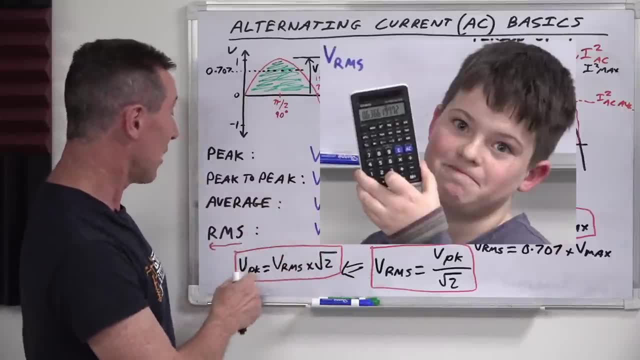 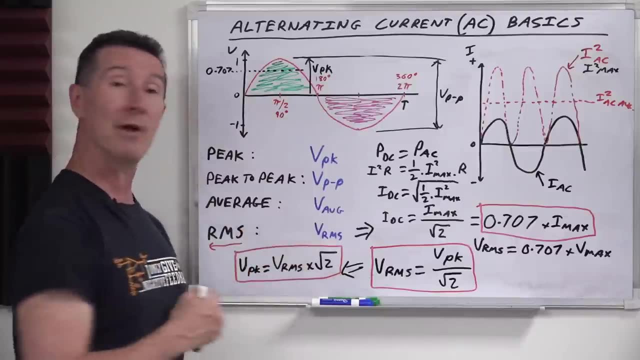 but square root of two will give you a more precise answer. So and that, if you just rearrange that formula V, peak, peak voltage equals the RMS voltage times the square root of two, Easy, And there's other formulas which derive, you know. 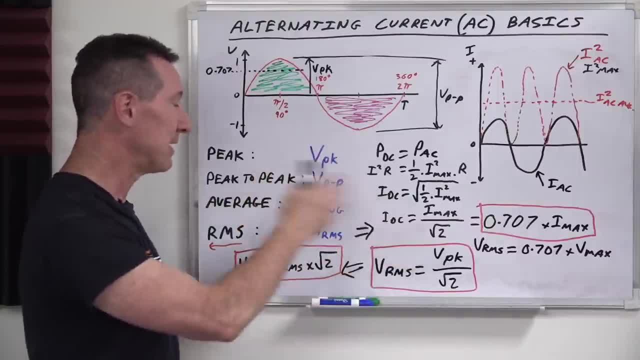 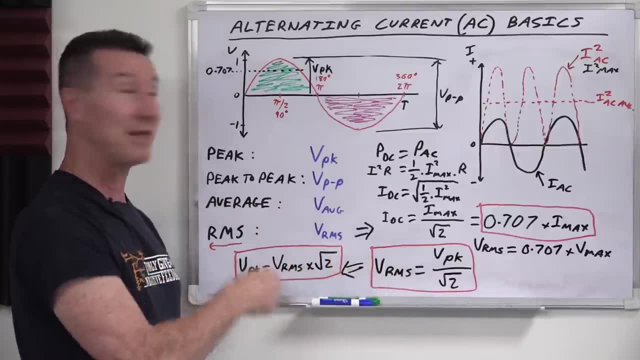 you can go directly from volts RMS to peak to peak or peak to peak to RMS or whatever You know. there's various combinations of these, But if you just remember well, if you remember one of them, you can derive the other. 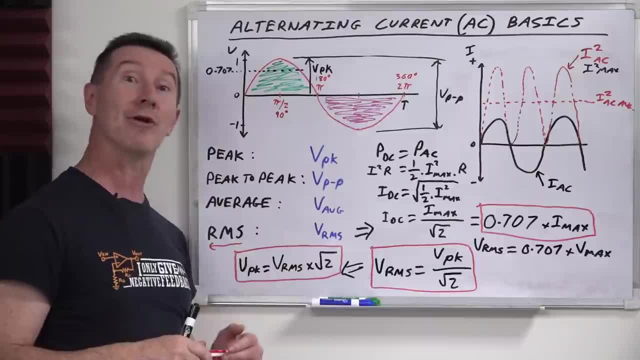 and then you can derive the peak to peak from the peak, et cetera, et cetera. Now we've only looked at ideal sinusoidal waveforms. but what if you've got, I don't know, a sawtooth waveform like this? 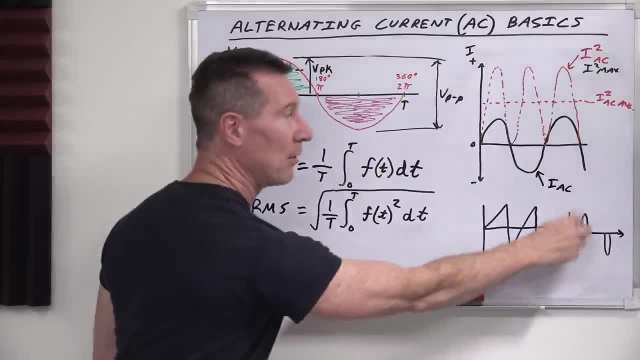 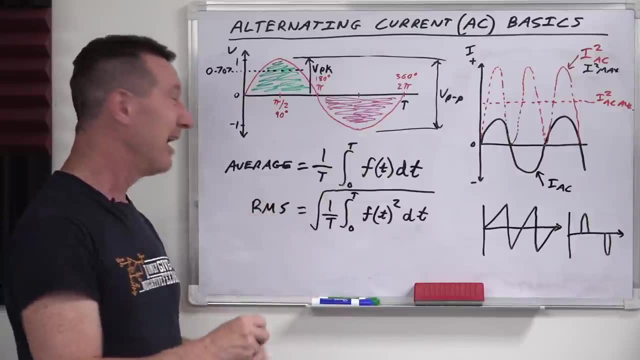 or you've got like a high crest factor- we might go into that- a waveform like you know, a current waveform like this. How do you get that? Well, we start looking at integrals, and this is where you get a little bit more advanced calculus. 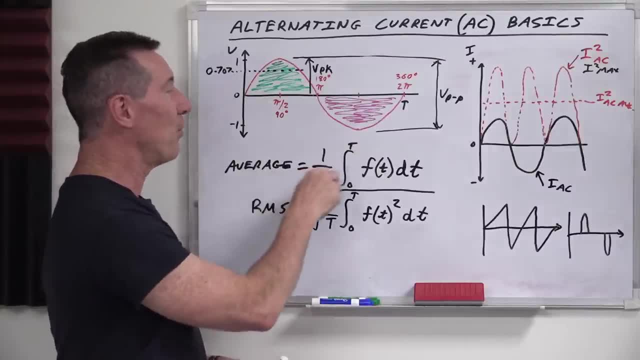 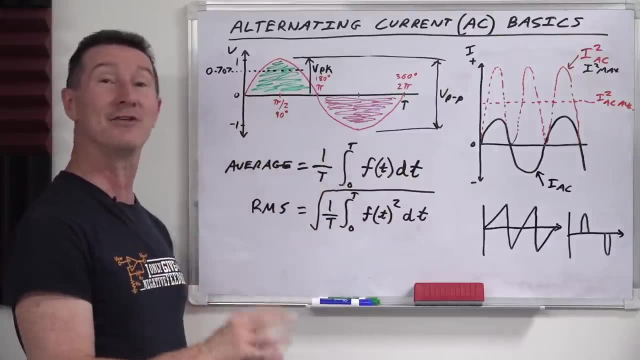 which we don't really want to go into here. So the average value 1 on t, the integral from 0 to t and then the function of that, And we won't go into the details. You can do this yourself. 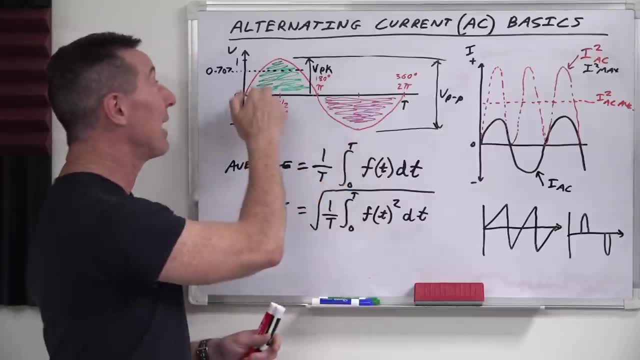 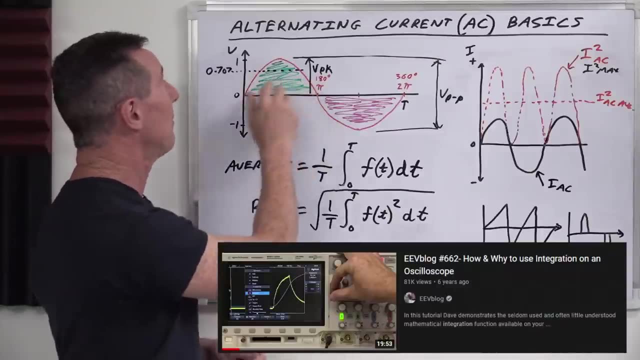 But it's basically an integral is just the area under the curve, And I've done a practical video, I believe, showing this somewhere. I'll try and link it in on an oscilloscope. The integral is just the area under the curve. 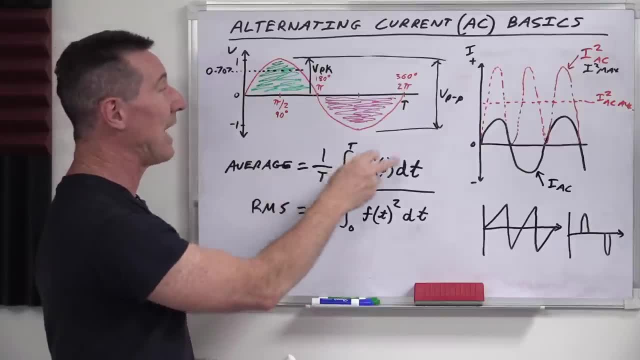 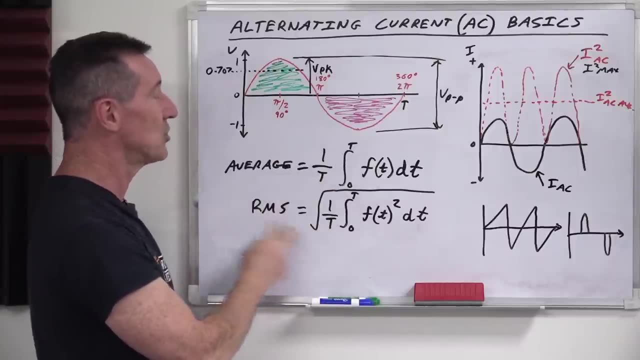 So it's exactly what we did before, but you can actually do the average derive. you can derive the average formula we did before using integrals and stuff. But anyway, it's that And the RMS version of it is simply the square root with the squared in there. 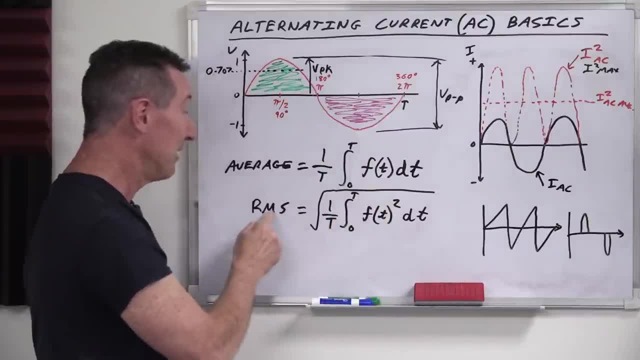 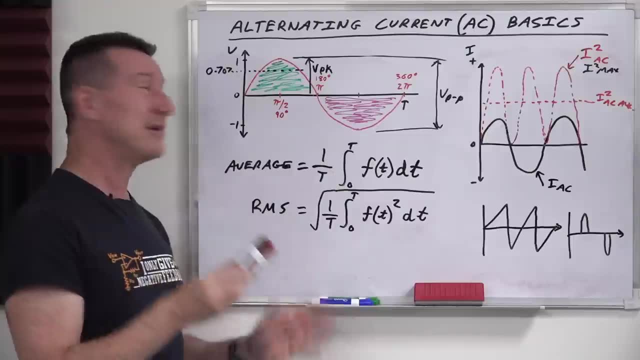 It's exactly the squared factor, the mean factor and then the square root in there. So anyway, we won't go into details. It's basically just getting the area under the curve. So you just have to get this area under the curve here. 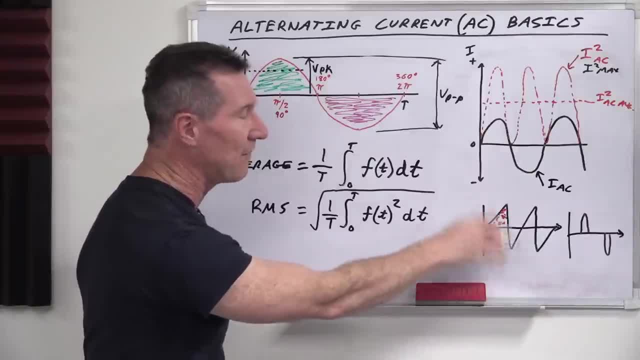 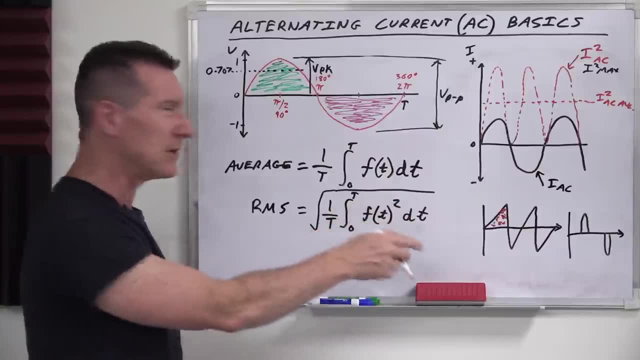 And you can do that using graphical methods. if it's just like a sawtooth waveform or something like that, Or even, you know, a pulse current waveform like that, like a poor power factor on a DC to DC converter, You'll get a waveform like that. 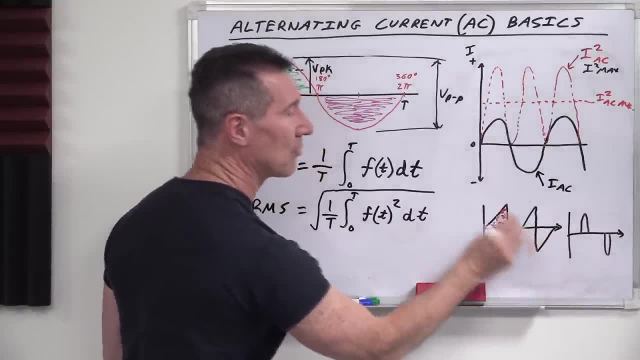 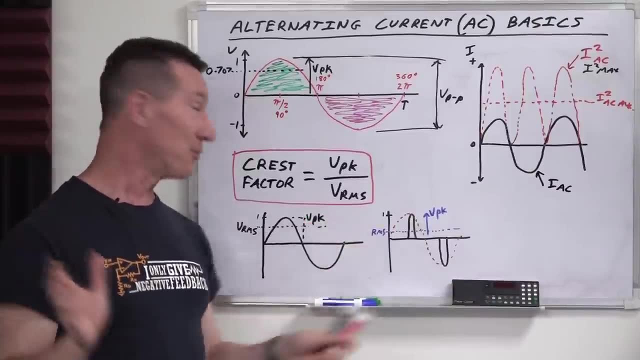 I've shown that in previous videos. You can do these actually using graphical methods, or you can do it using differential calculus. Now, the absolute last thing we're gonna look at- I swear for this video anyway, just to round this off- is what's called crest factor. 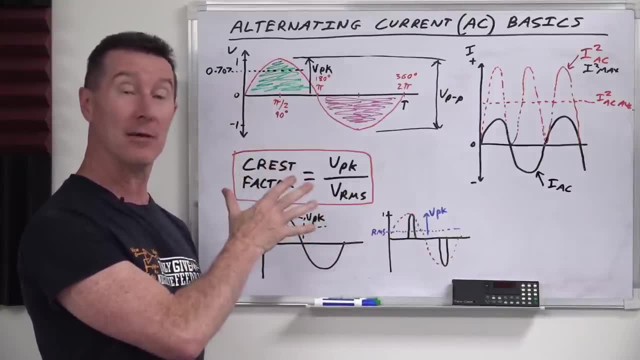 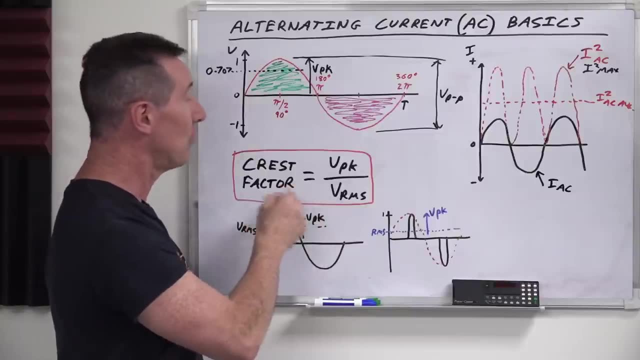 And this is important for RMS- true RMS measurement. you might get on your multimeter, for example. This is also known as peak factor As well. This is also known as peak factor As well, And the crest factor or peak factor is the peak on the RMS. 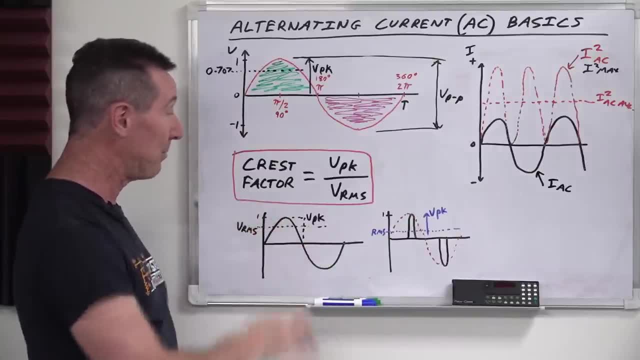 So if we've got our waveform here, obviously we've got our peak value up like this easy and our RMS value is gonna be 0.707 times the peak there that we've seen and that gives a crest factor of 0.414.. 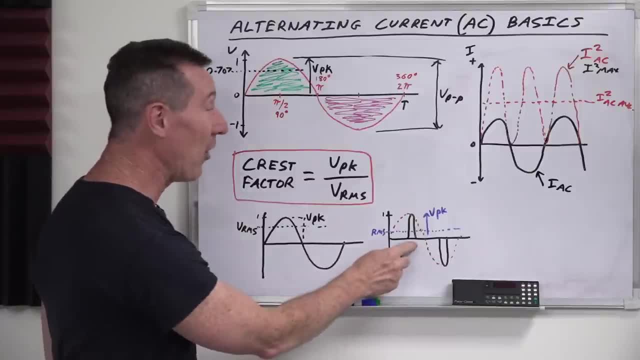 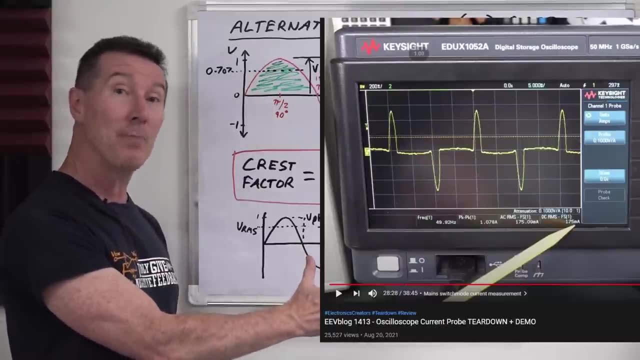 Beauty, No worries. But if you've got a horrible waveform like this, like the sine wave is like this. but you've seen this in videos- where you might have a a non-power factor corrected, mains power supply, for example, current peaks could be up like this. 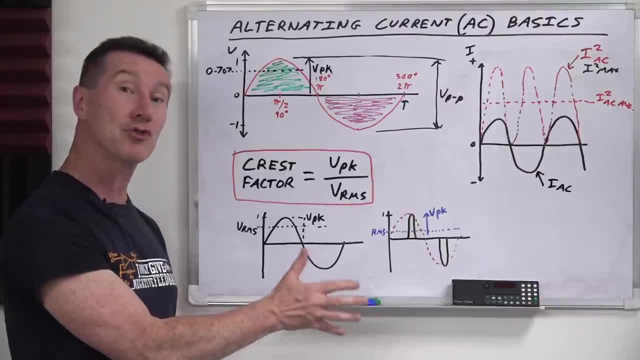 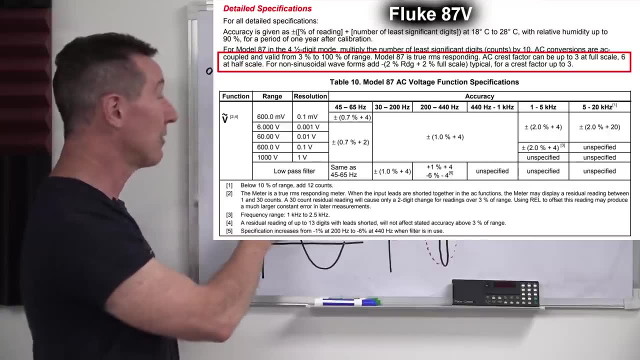 And if you're trying to measure, say, with your multimeter, using your true RMS converter, in your multimeter of this waveform like this, if it has a too-higher, too-higher crest factor, like this, your true RMS converter won't be able to. 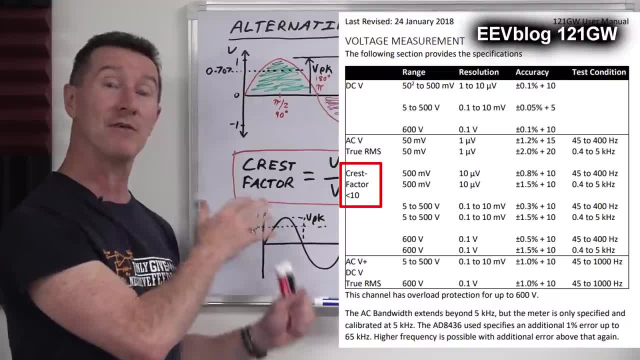 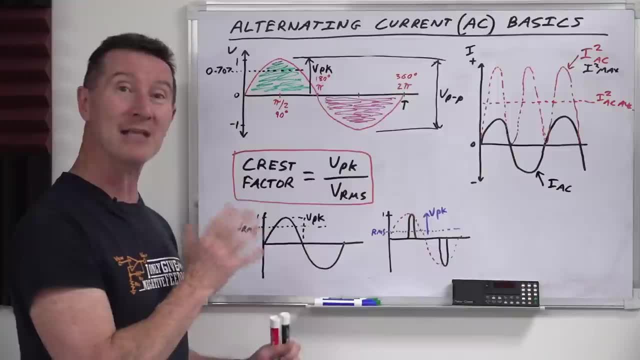 handle it And you'll often find the maximum crest factor value in the data sheet for your meter or your true RMS converter chip measurement system, whatever it is. it is So there's a maximum. you know they can't tolerate an infinitely small pulse like this. 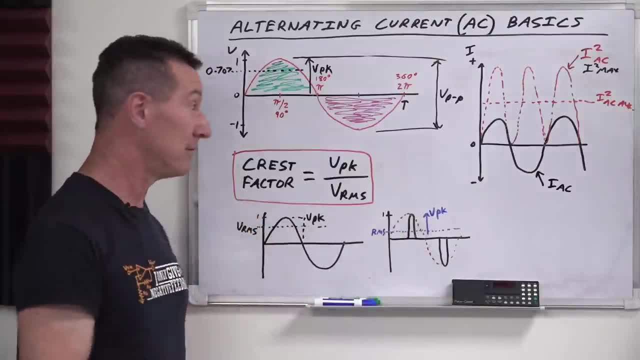 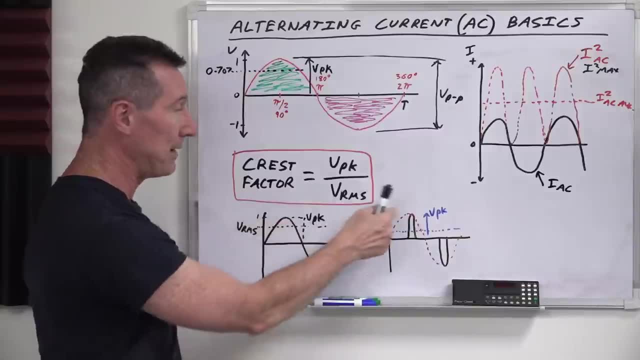 There's going to be a point where they come a gutter and just go. I'm going to give you know I'm not going to give an accurate value, I'm going to read low So you can see that the, in this particular case, the peak value might be absolutely identical. Say it's one between the two. 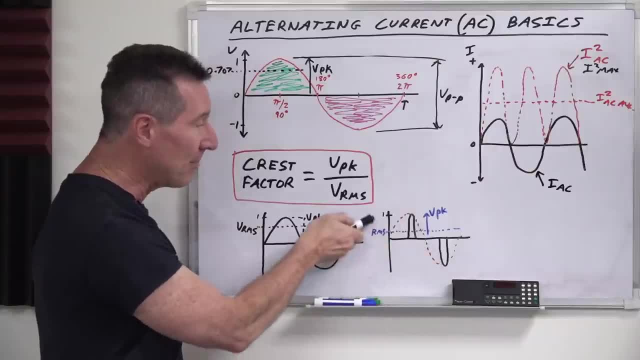 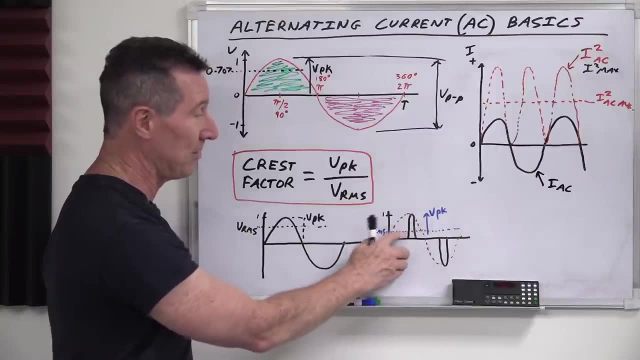 of them, but because it's much shorter, like this, the RMS value, of course, is going to be much lower. It's not going to be 0.707 anymore because there's no longer a perfect sine wave, So it could be, could be, you know, 0.2 or something, volts or something like that, So it's going to be one. 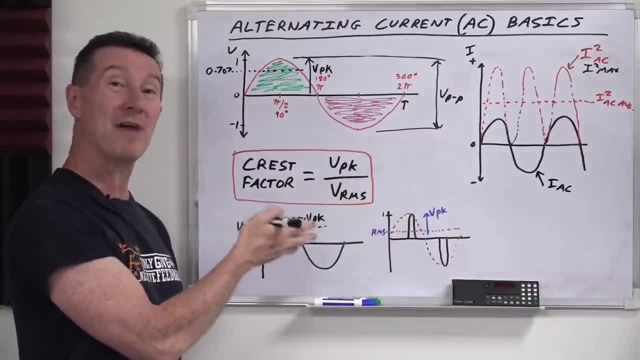 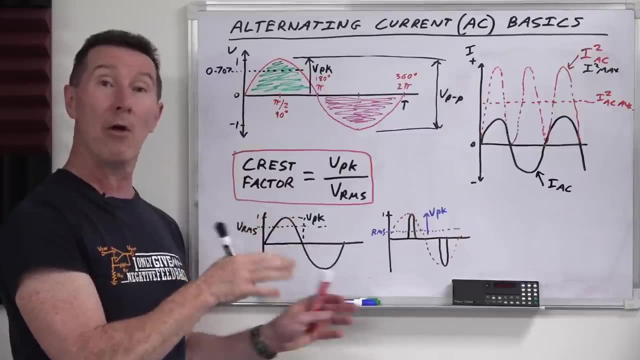 divided by 0.2,, for example, it's going to be a crest factor of five. And that that starts getting up there, towards where you know your true RMS converter multimeter, because there's different methods for RMS conversion which we won't go into. Maybe I've done that in another. 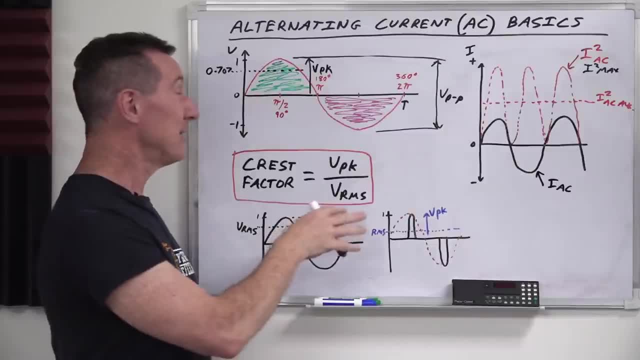 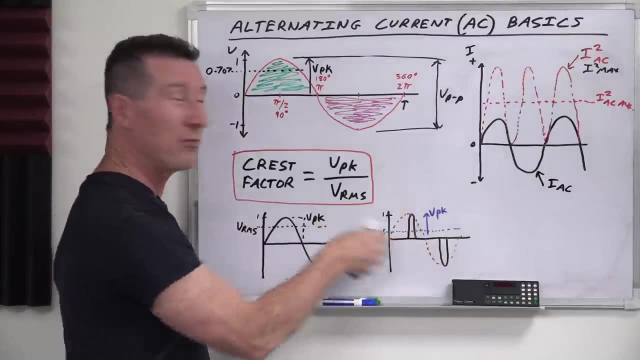 video. Don't know done so many videos And yet that's getting. you know, that's getting pretty high. So once this gets narrower and narrower and narrower, or the, you know the ratio it doesn't like. the waveform can be different, It can be any type of waveform, But the crest factor 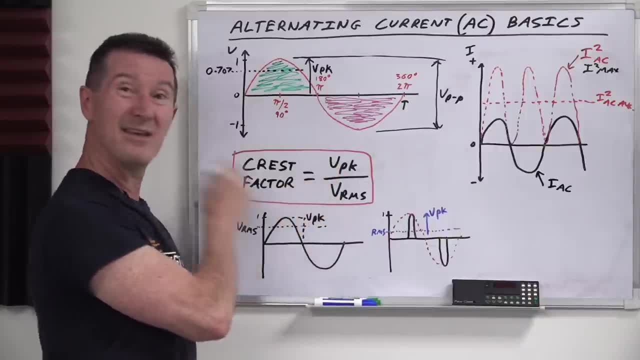 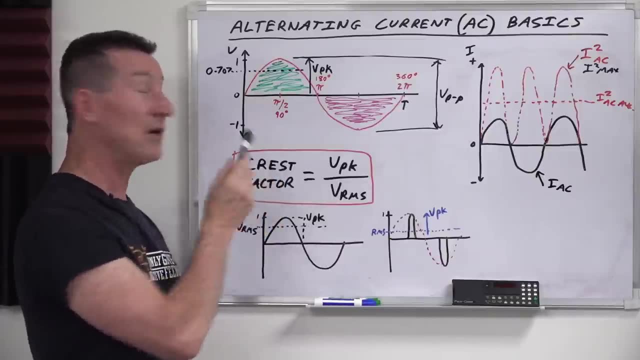 V peak on VRMS. if that's too high, then yeah, it screws up your RMS calculations And you need basically, you know better, faster sampling hardware for your RMS converter chip to actually measure it, Or you might have to go to some method that there's RMS converter chips that 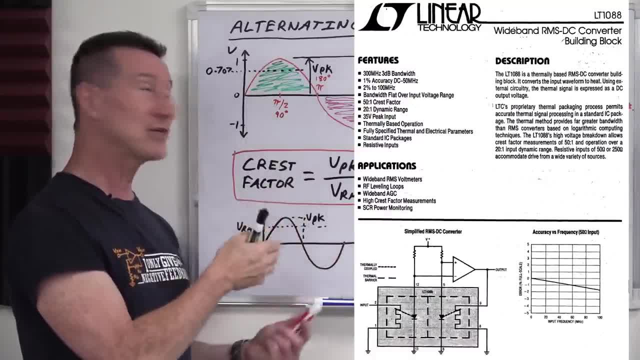 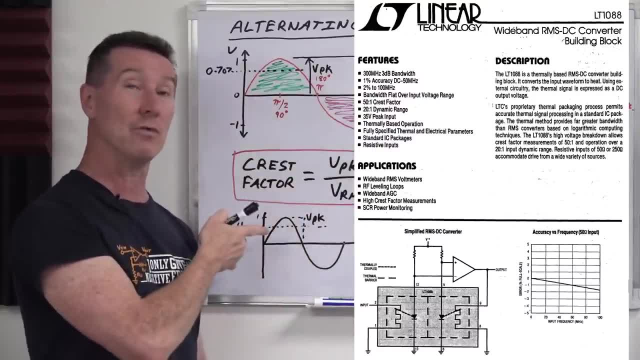 actually measure the heating in the resistor. So they don't actually, you know, do it sampling wise. They actually, like physically measure how much power is going to be in the resistor. That's old school, 1960s, 70s stuff. So I hope you found that introduction to AC useful, I know. 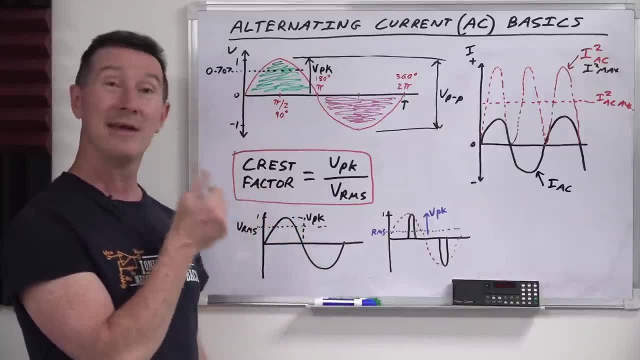 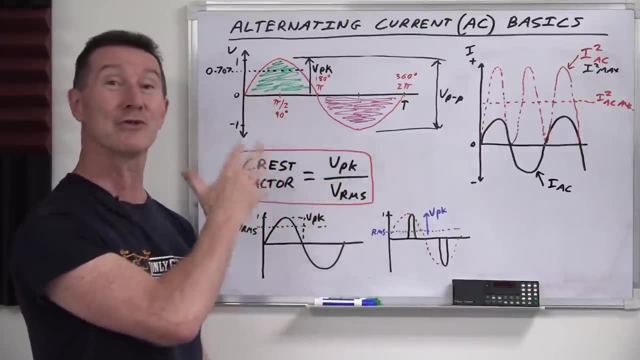 it's very long and there's lots of stuff to cover. I could have broken it up maybe into smaller videos, but there's a lot more to come. We haven't even gotten into other stuff like transformers and circuit theory and all sorts of other stuff and AC, ohms law and all the rest of it, But yeah, 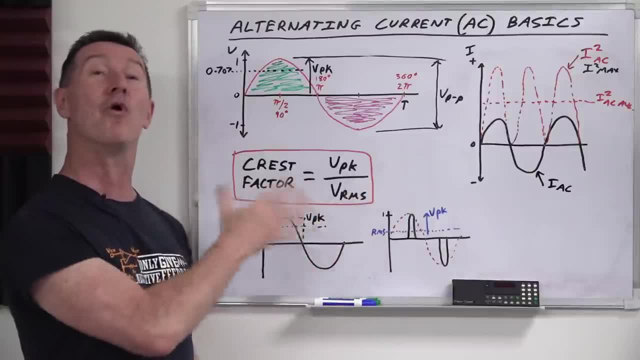 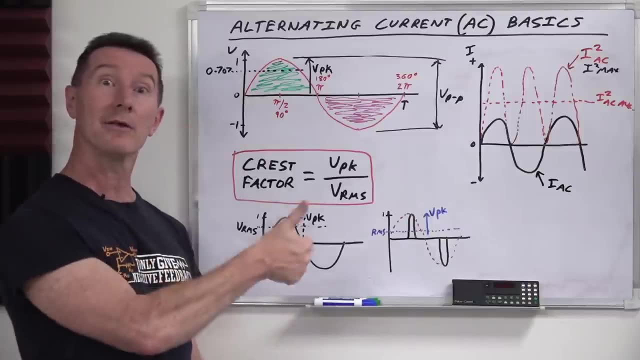 complex numbers and things start coming next. but this will all be in part of the AC circuit theories circuit theory series. There you go. If you liked it, give it a big thumbs up. As always, discuss down below. Catch you next time.